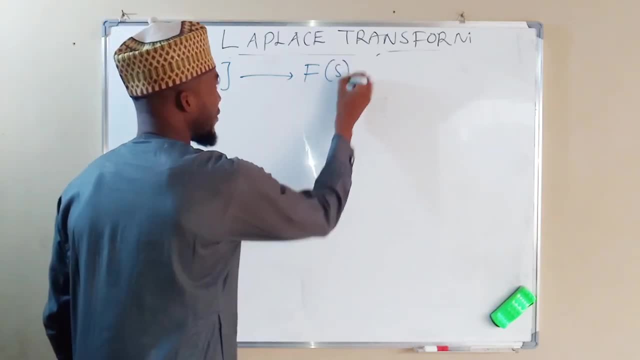 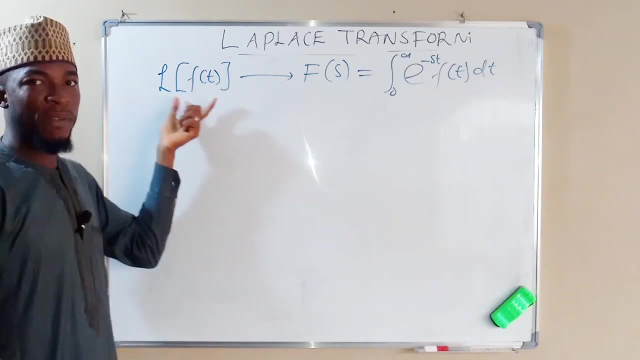 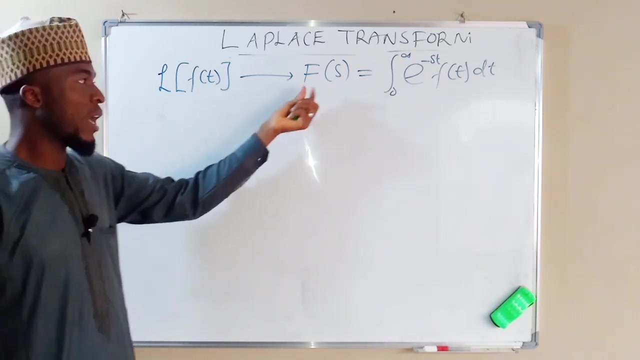 entirely different function, say f of s, And this f of s can be obtained. So here we have a function of t, but it transform it into another function which is entirely different from this function. And to obtain this function we have to take the integral from zero to infinity of exponential. 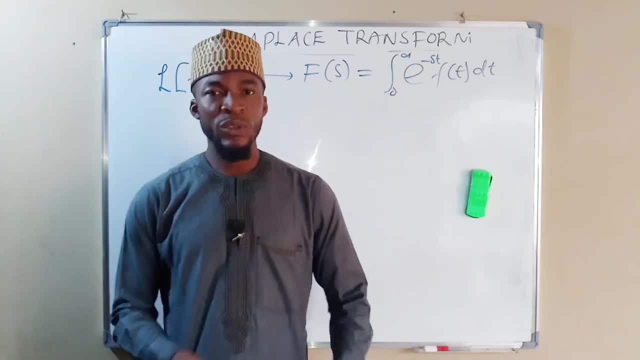 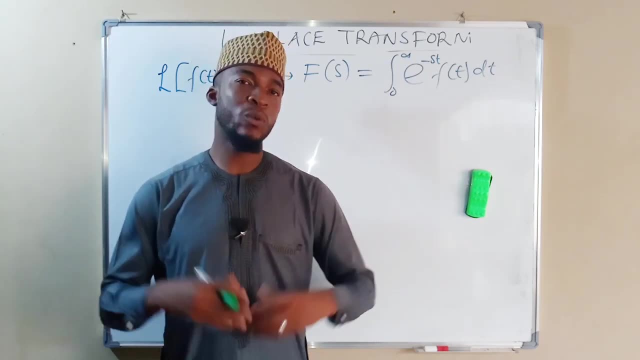 negative st times the function with respect to t. So in this tutorial we are going to derive five fundamental functions of Laplace transform. First of all, we are going to learn how to derive five fundamental equations that will help us in solving subsequent problems. So the first one. 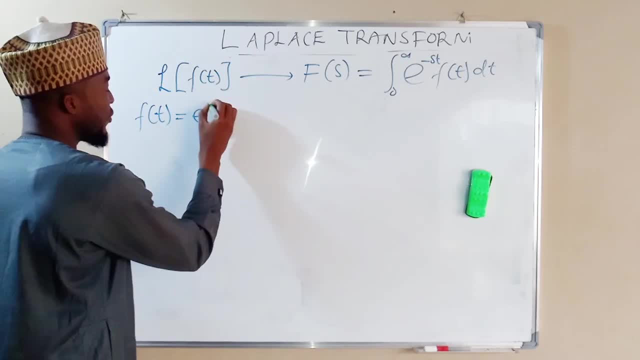 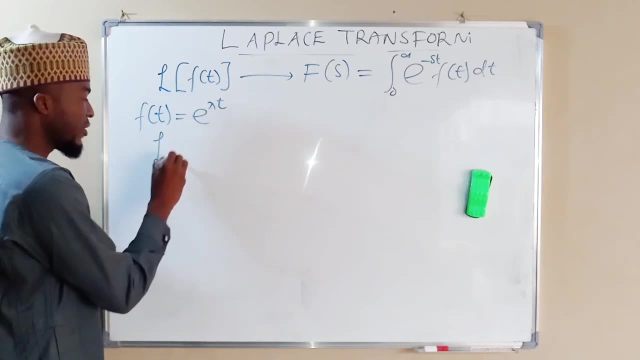 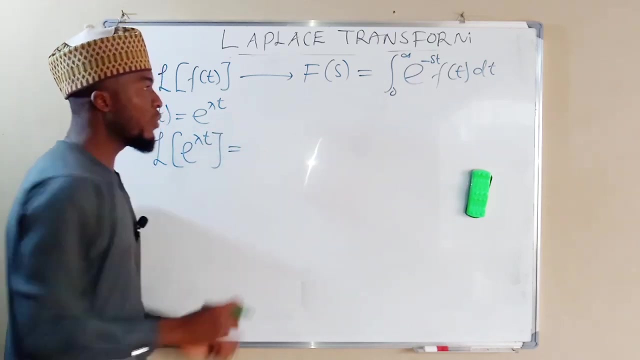 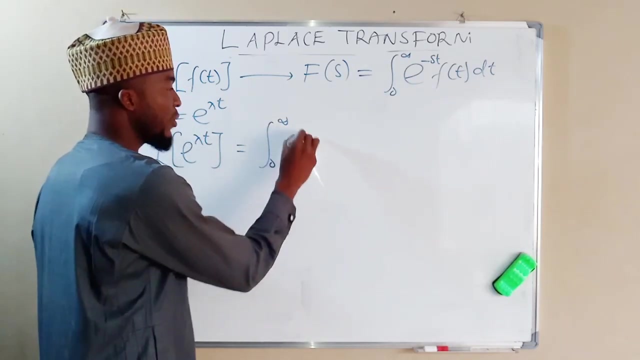 let f of t equals to exponential lambda t, where lambda is any constant. So therefore we have the Laplace transform of exponential lambda t, which is equal to. we are going to now substitute this information into our integration: The integral from zero to infinity exponential negative st times the function f of t, which is now. 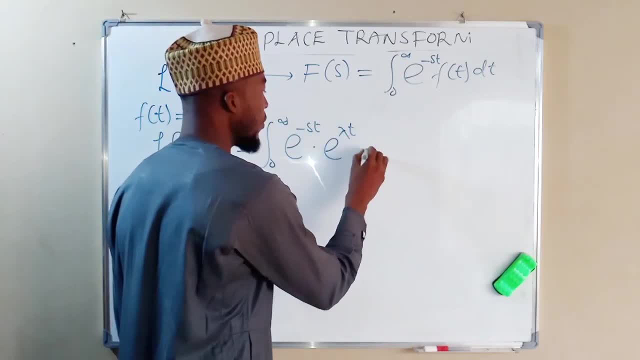 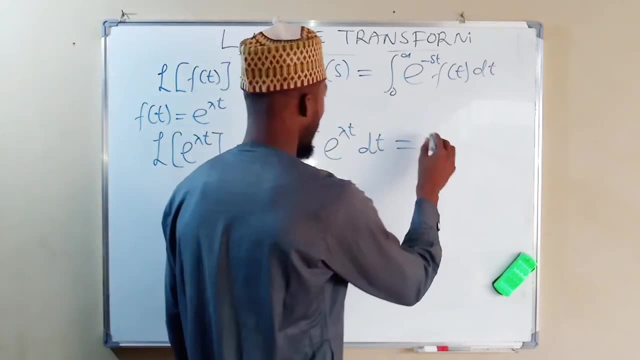 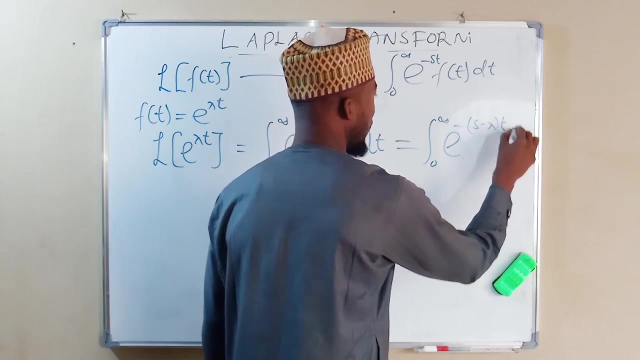 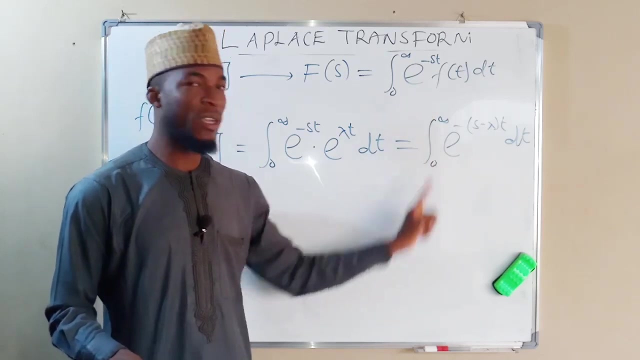 exponential lambda t with respect to t. This is equal to: because we have common base, we can add the index together, The integral from zero to infinity of exponential negative s minus lambda t with respect to t. Now what we are are going to do: we are going to integrate this function and substitute our lower and upper bounds. 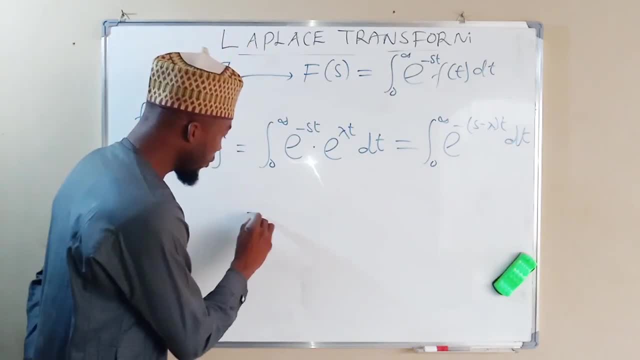 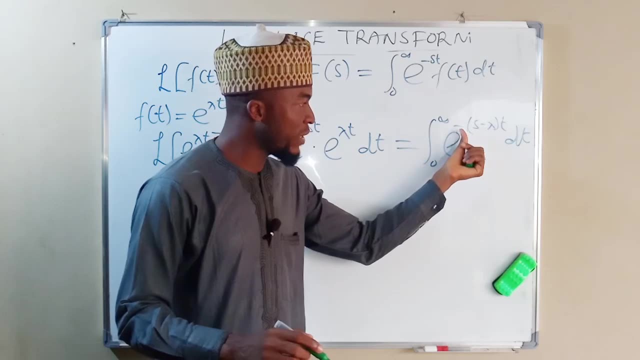 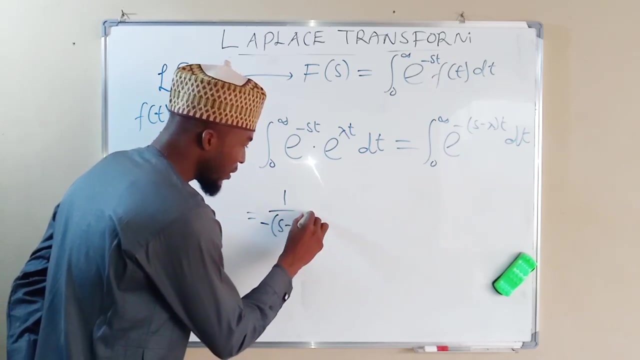 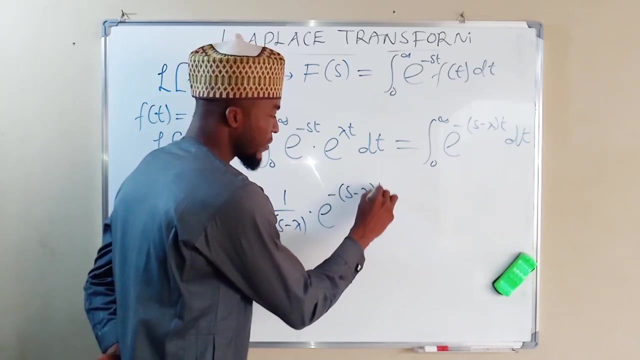 if we integrate this function, we are going to get 1 divided by the derivative of the index with respect to t, which is now going to be negative s minus lambda negative s minus lambda times, exponential negative s minus lambda t, and we are going to substitute our lower and upper bound. 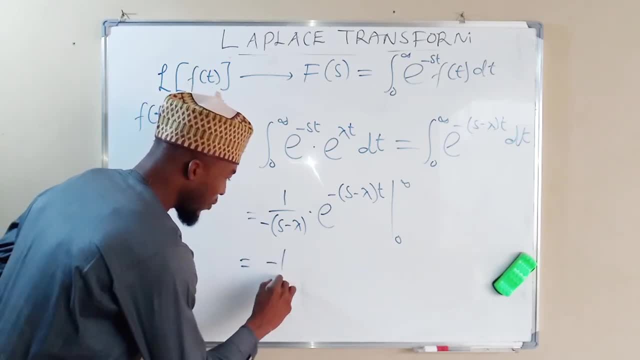 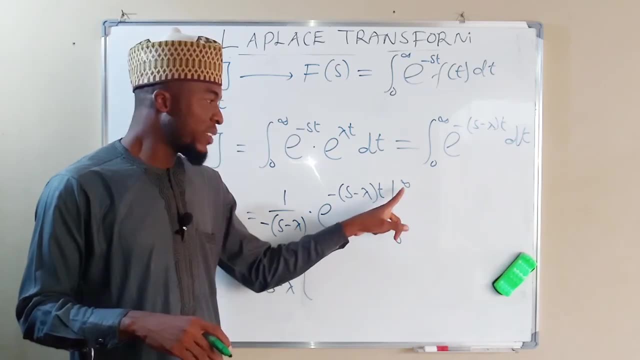 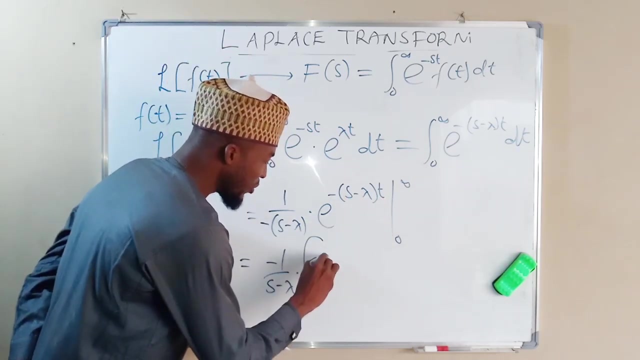 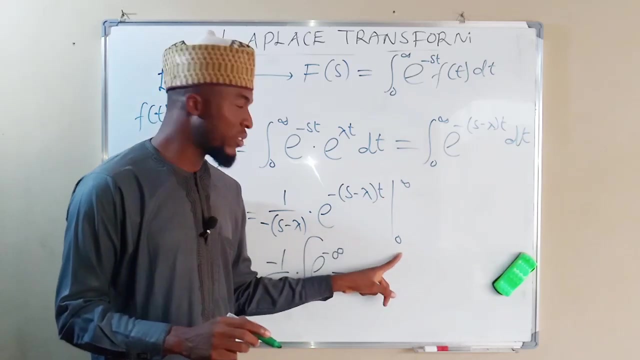 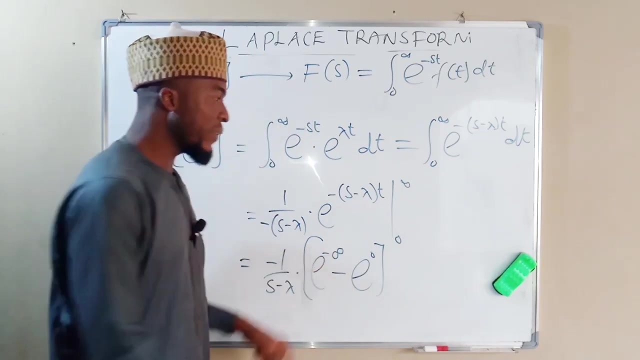 this is equal to negative 1 over s minus lambda times. so if t is infinity, the whole of this term, multiplied by infinity, is going to be infinity. so we have exponential negative infinity minus the lower bound, which is now. if t equal to zero, the whole of this will be zero, exponential zero. here we have exponential negative infinity, which is: 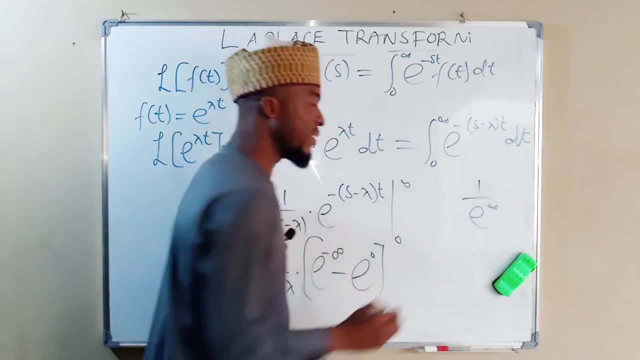 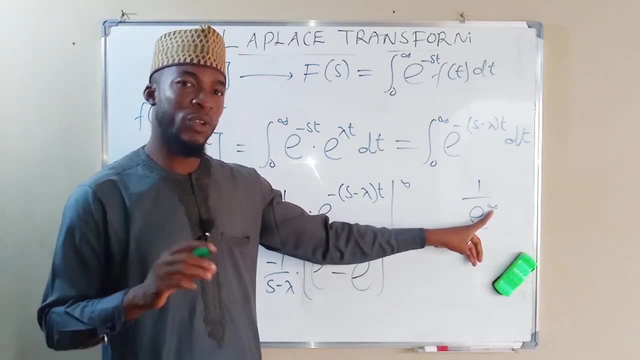 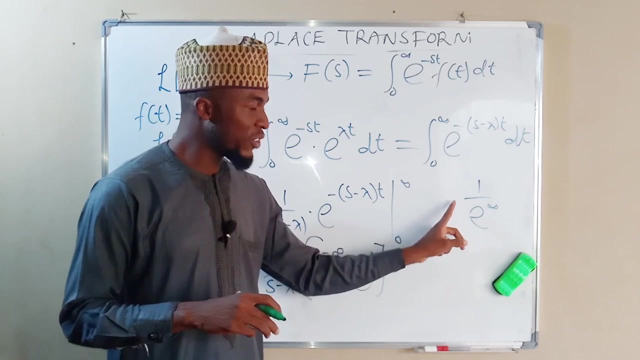 the same thing as 1 divided by exponential infinity. so we are going to apply the aspect of limit in this substitution because we don't know any number called infinity, but we know that it is a very large number. so if we apply the aspect of limit in this expression, 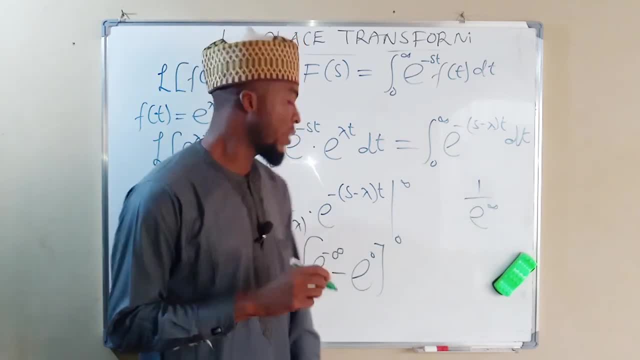 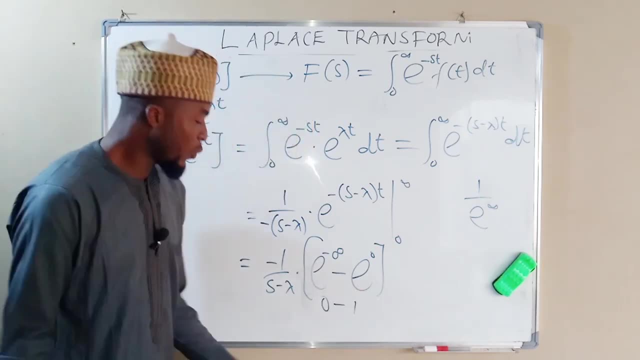 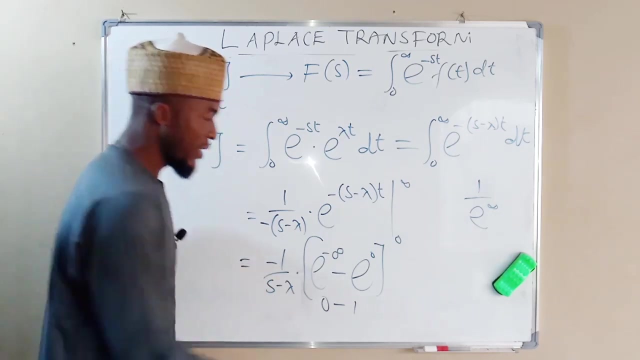 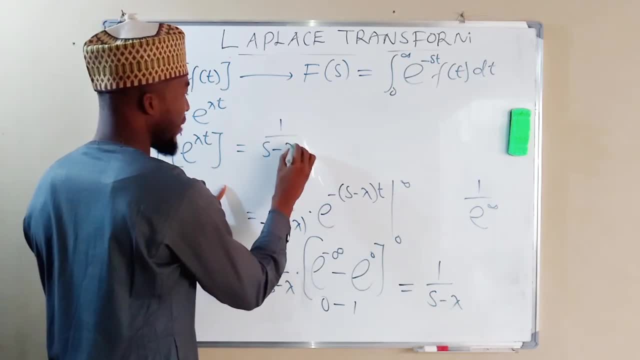 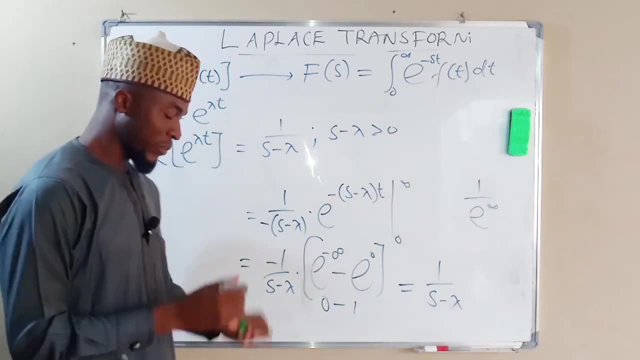 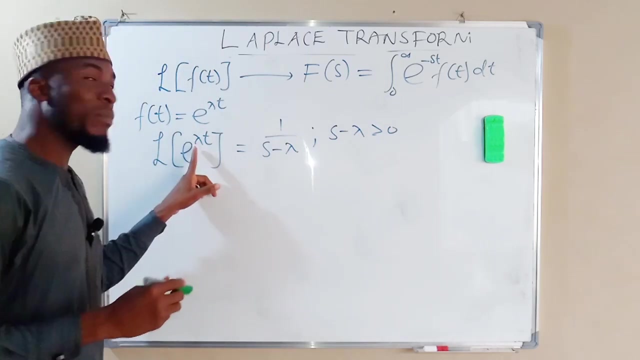 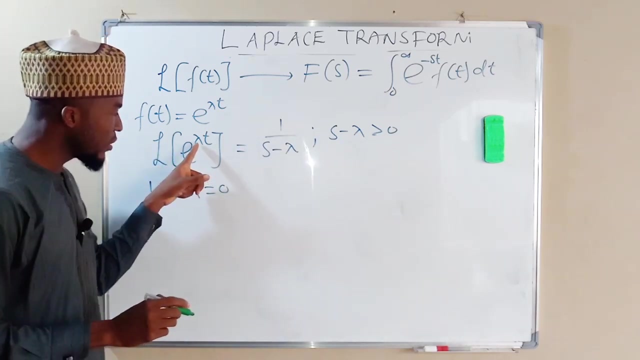 this is just one divided by s minus lambda, for s minus lambda greater than zero. so this is our first formula. now to obtain the second one, since lambda is constant, let lambda equals to zero. if lambda equals to zero, So 0 times t will make it 0, and exponential 0 is 1.. 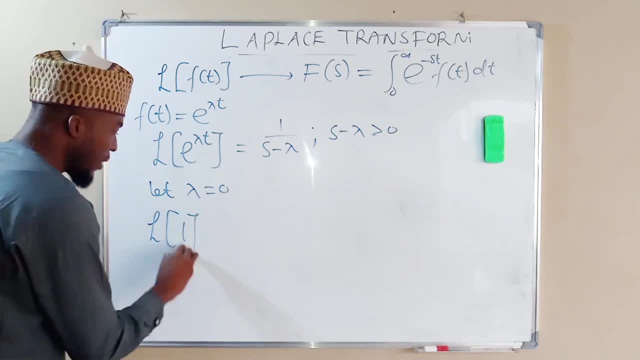 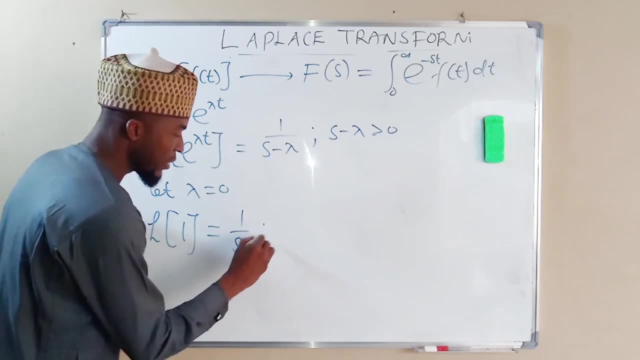 So we have Laplace transform of 1, which is going to be equal to. since this is 0, we are going to only have 1 over s 4s greater than 0. So now we have obtained two equations, 1 and 2.. 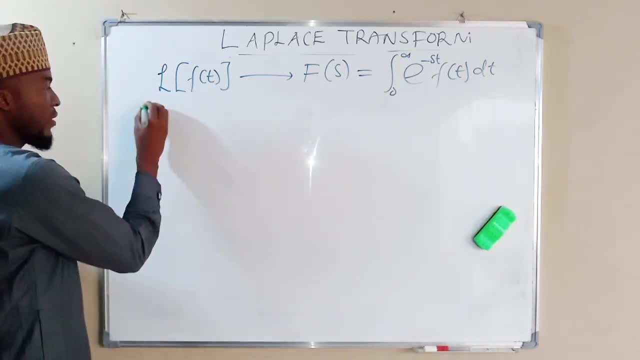 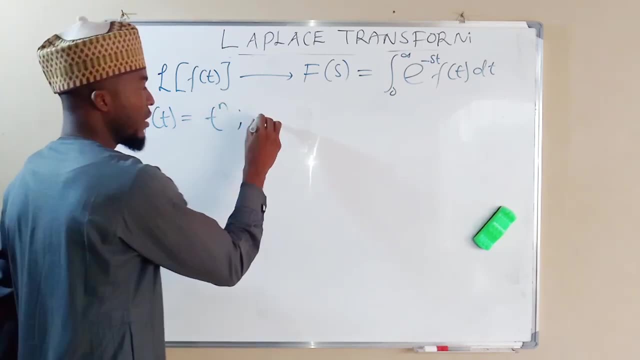 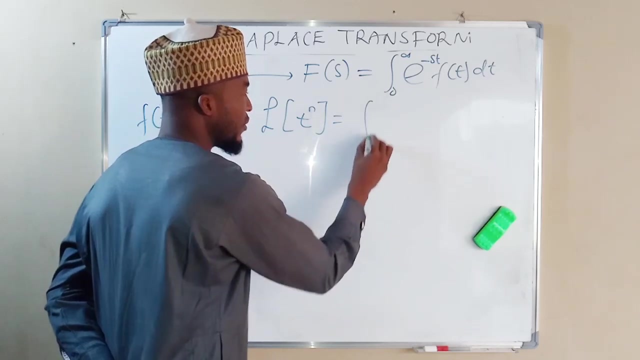 Now let's find the third one. Now suppose f of t equals to t to the power of n. The Laplace transform of t to the power of n will now be equal to the integral, from 0 to infinity, of exponential negative st times t to the power of n with respect to t. 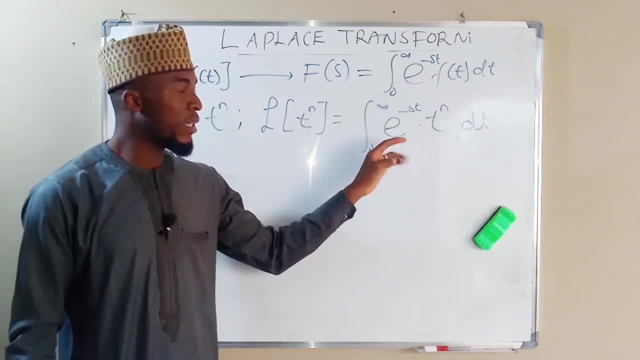 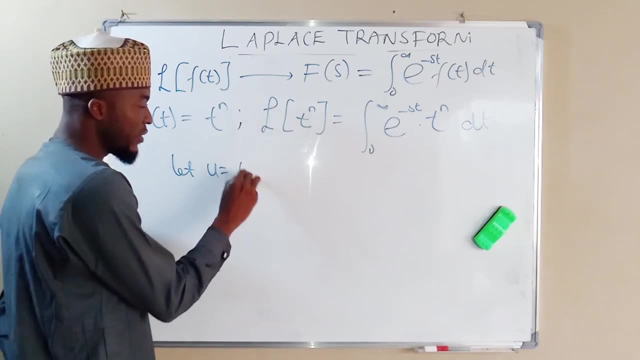 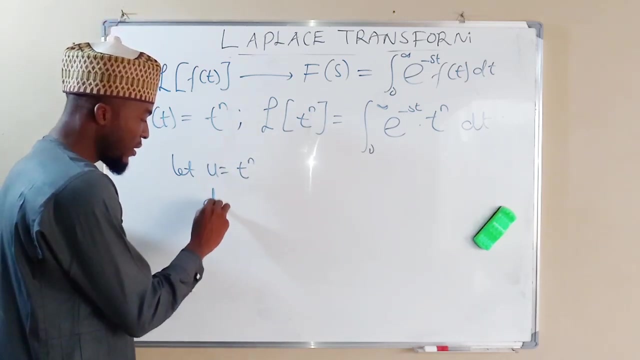 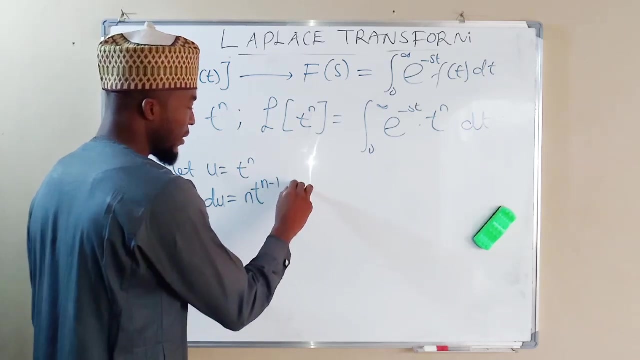 These two functions are different. therefore we are going to apply integration by part here. So let's Let u equals to t to the power of n. If we take the derivative of u with respect to t, we are going to obtain du equals to n, t to the power of n minus 1 dt. 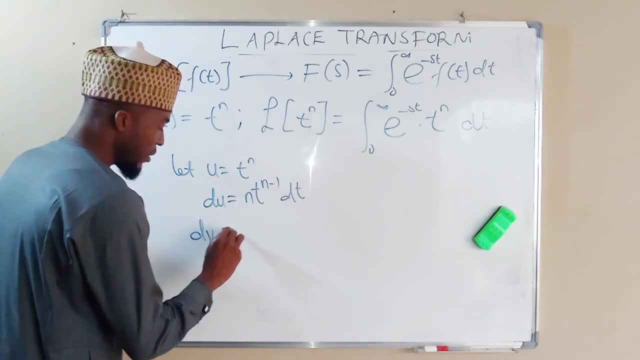 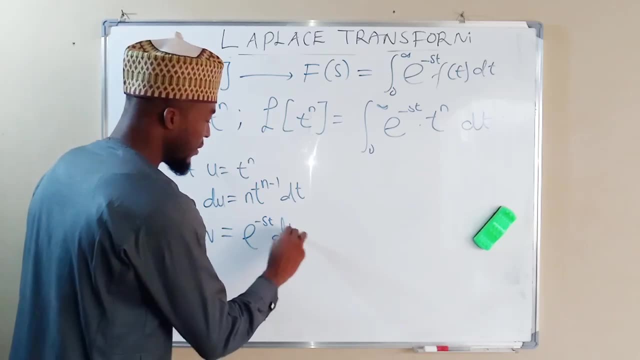 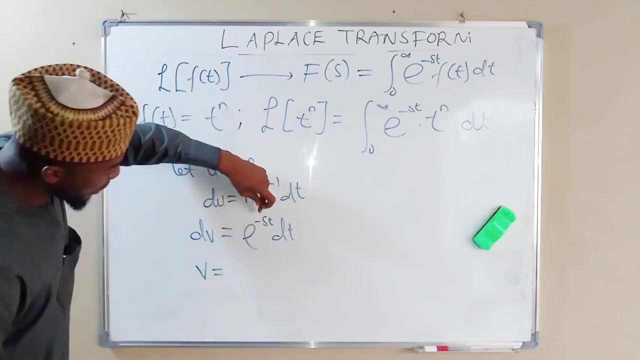 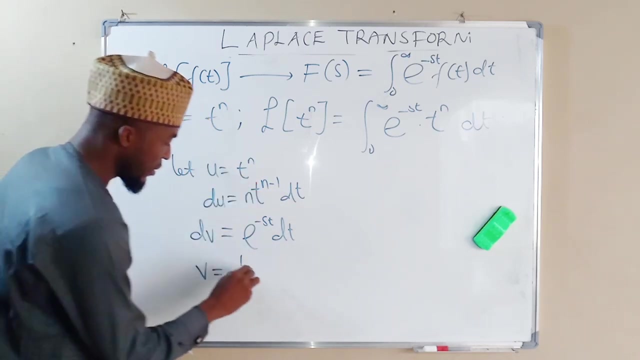 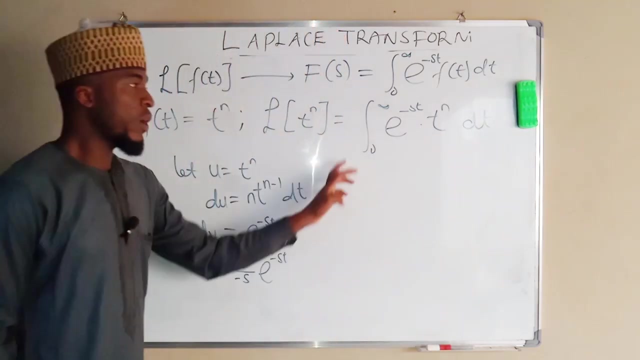 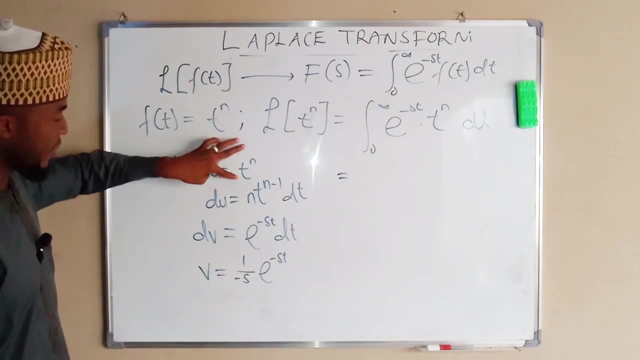 dv is equal to exponential negative st, dt. To find v, we are going to integrate both sides and v will now be equal to 1 divided by the derivative of this index, which is just negative s times exponential negative st. So now this integral will be equal to uv, and you know that u is t to the power of n and v is equal to this. 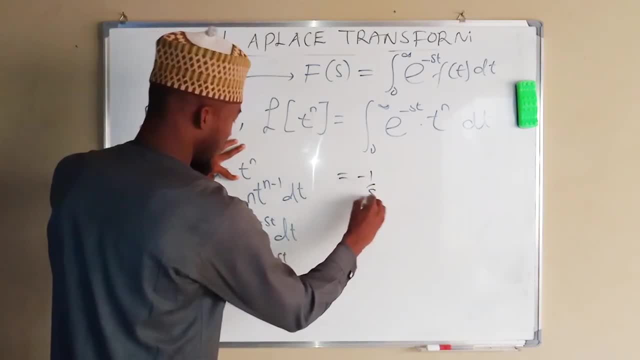 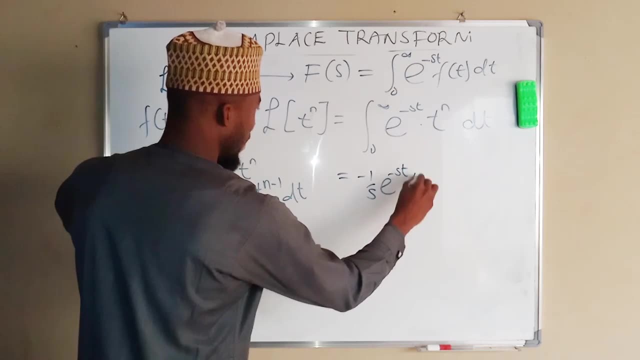 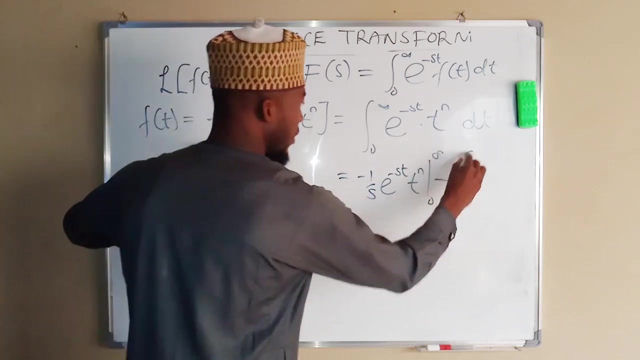 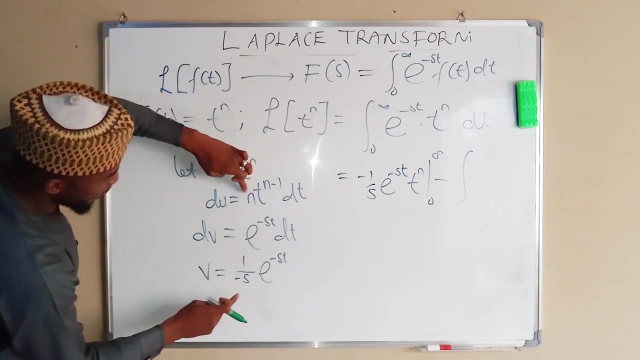 So we can say negative 1 over s, exponential negative st times t to the power of n, our limit from 0 to infinity. then, minus the integral of vdu, v is this and du is this, and we have constant n and 1 over negative s which we can factor out. 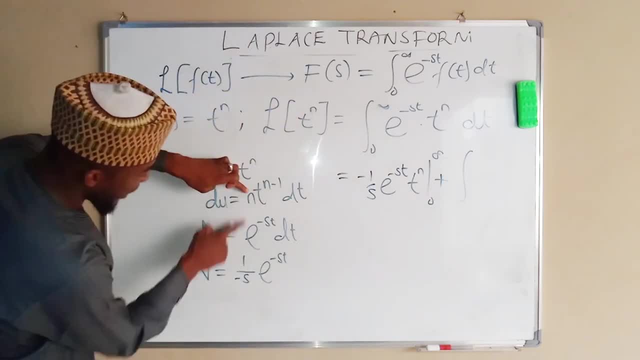 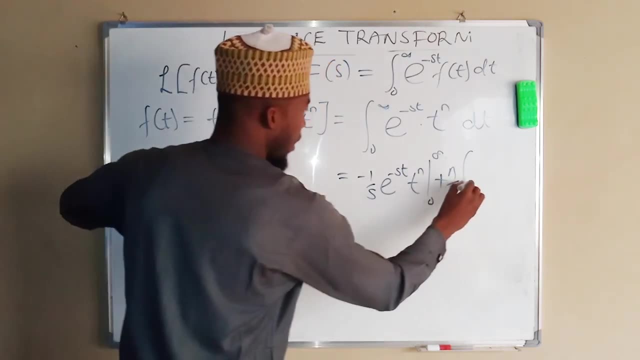 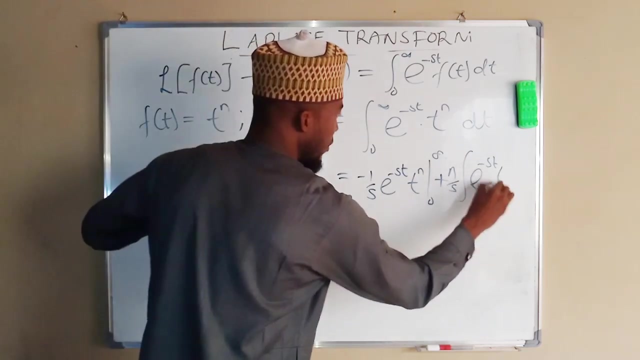 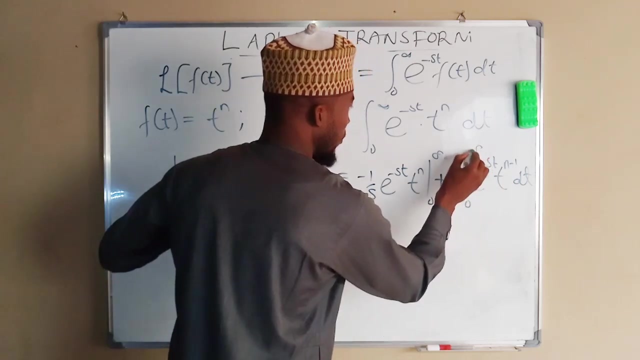 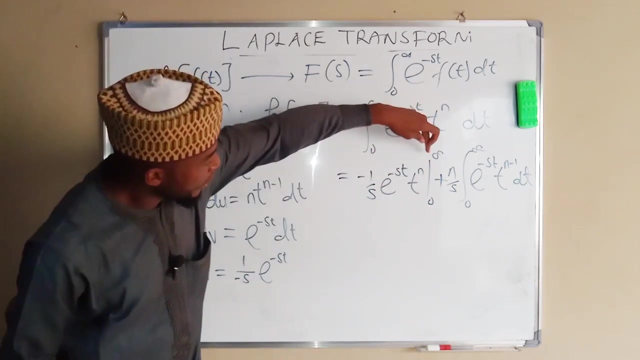 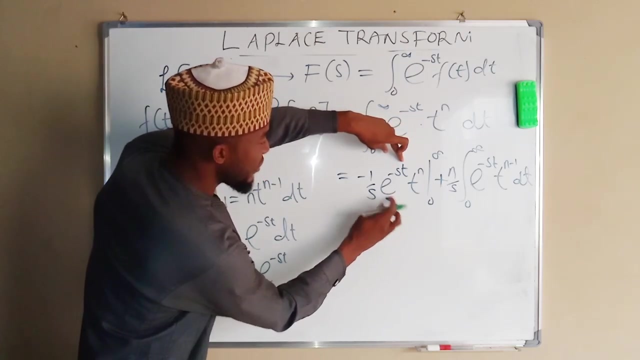 And this negative will change this to positive, and we have n over s. Then inside we have exponential negative st times: t to the power of n minus 1 dt, from 0 to infinity. Alright, so if we substitute, So if we substitute this limit, we can see that as t approaches infinity here the whole of this will be 0, because this is 0 times. this will make it 0. 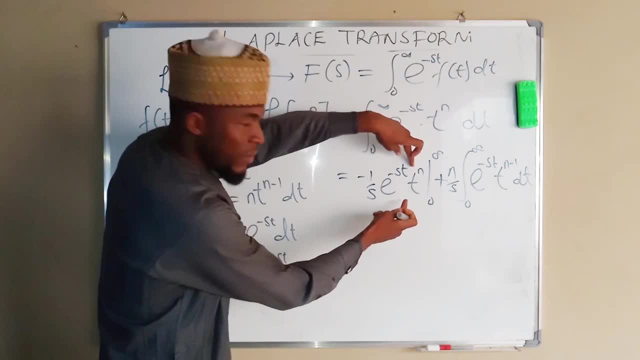 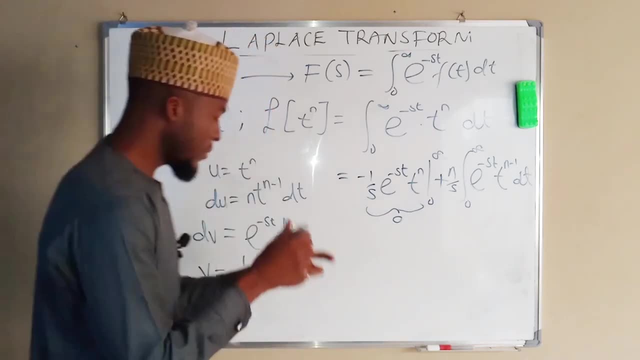 And if t is also 0,, you see, 0 to the power of n is 0, times the whole of this is 0. Therefore, the whole of this is equal to 0, we are only left with this. So now let us continue. 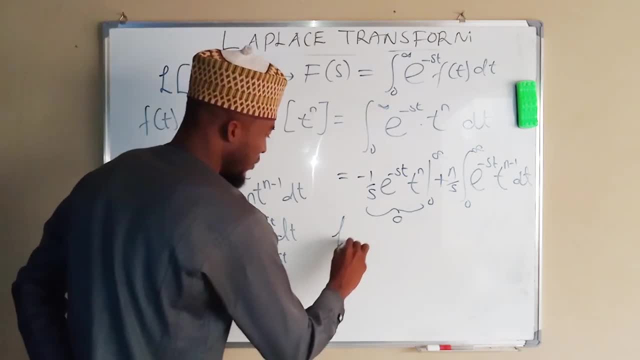 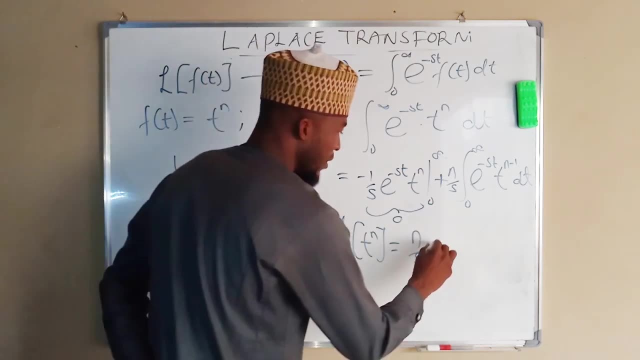 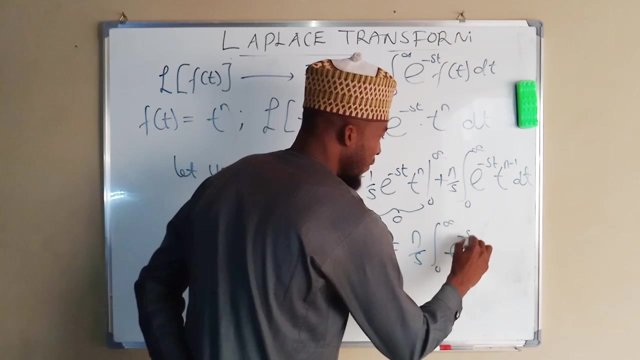 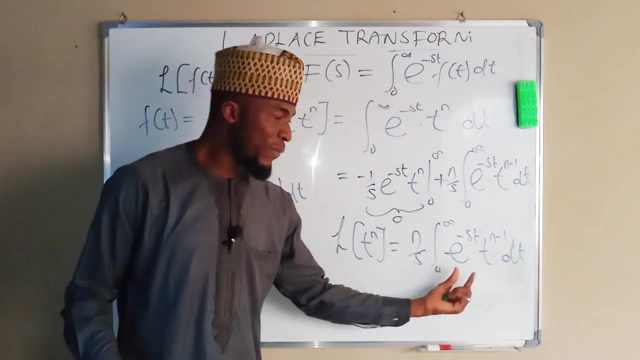 Therefore we can say the Laplace transform of t to the power of n, It is just equal to n over s, the integral from 0 to infinity of exponential negative st, t to the power of n minus 1, dt. But if you look at this function it is just the same thing as Laplace transform of t to the power of n minus 1.. 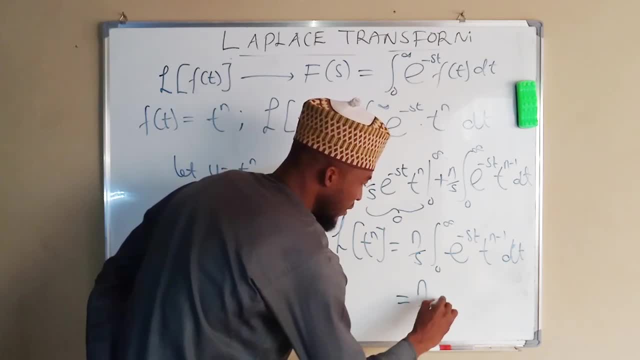 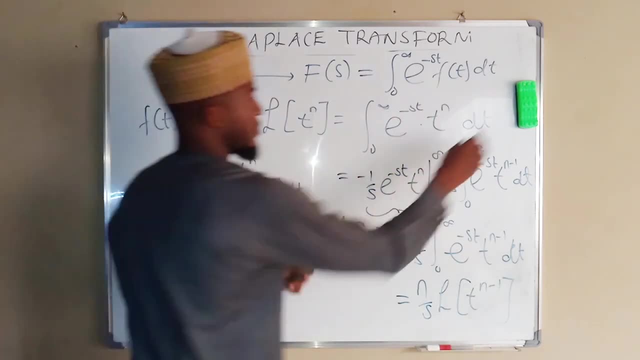 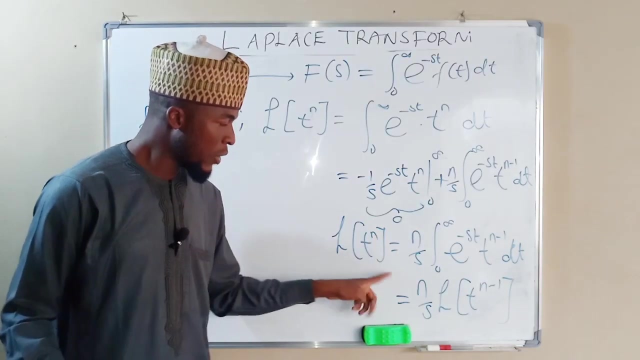 Therefore we say: this is equal to n over s The Laplace transform of t to the power of n minus 1.. There is something logical here. When we take the Laplace transform of t to the power of n, we got n, this n over s times the Laplace transform of t to the power of n minus 1.. 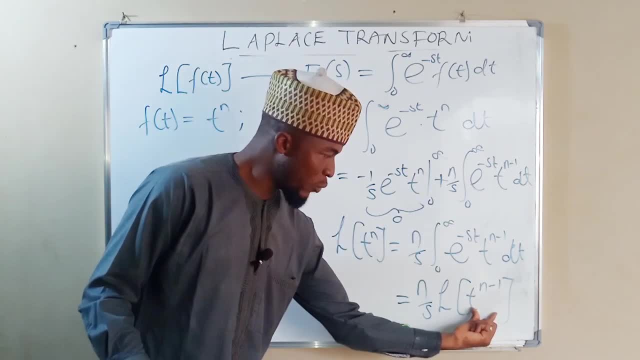 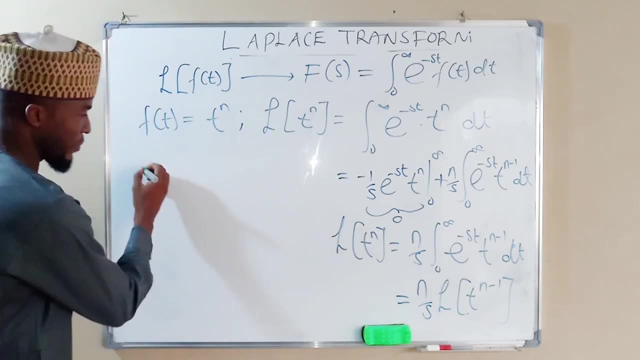 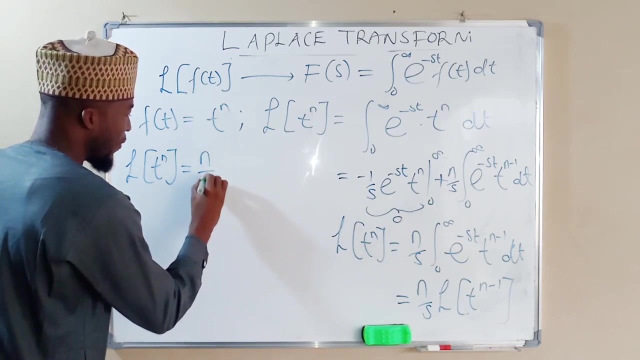 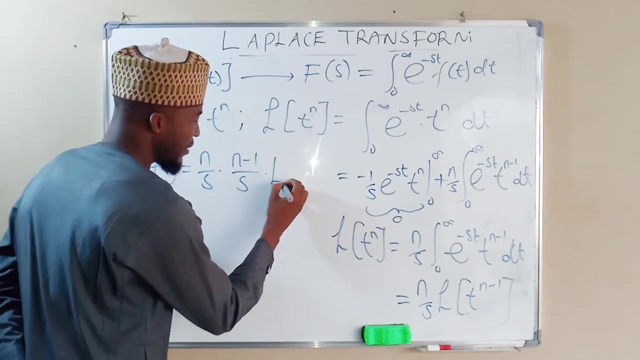 Therefore, if we take the Laplace transform of this again, we are going to get n minus 1 over s times Laplace transform of n minus 2.. So we say Laplace transform of t to the power of n will now be equal to n over s times n minus 1 over s. again times the Laplace transform of t to the power of n minus 2.. 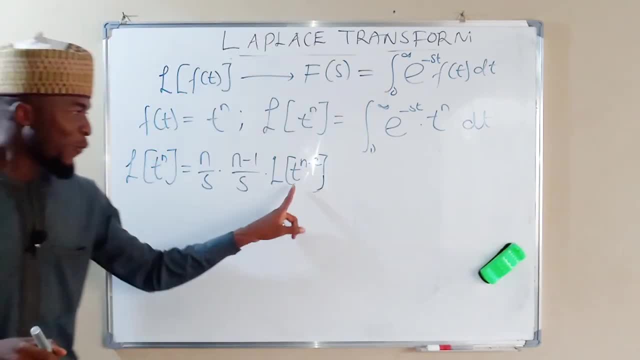 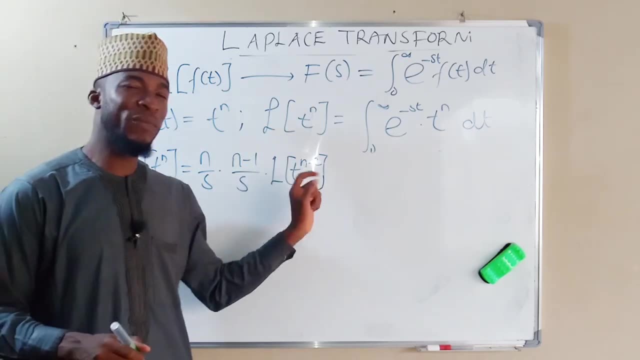 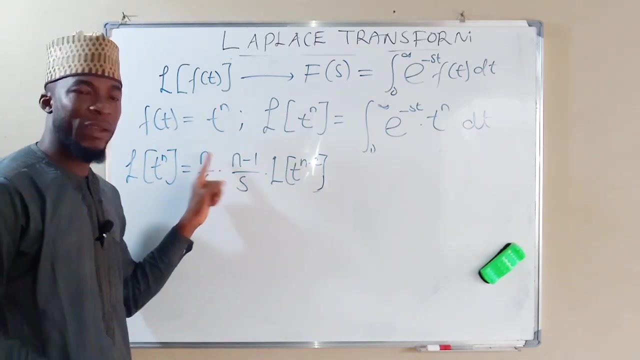 If we take again the Laplace transform of this, we are going to get n minus 2 over s times the Laplace transform of t to the power of n minus 3.. You can see that this is just reducing by 1, by 1, which defines n factorial. 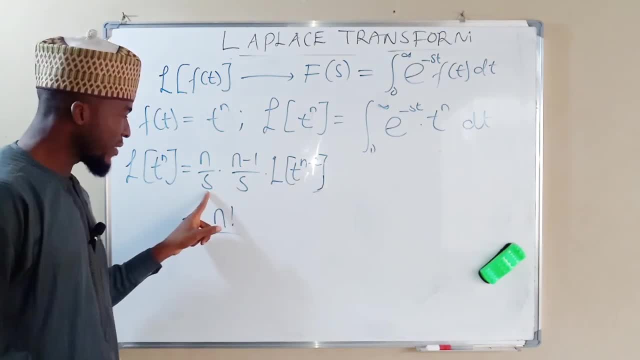 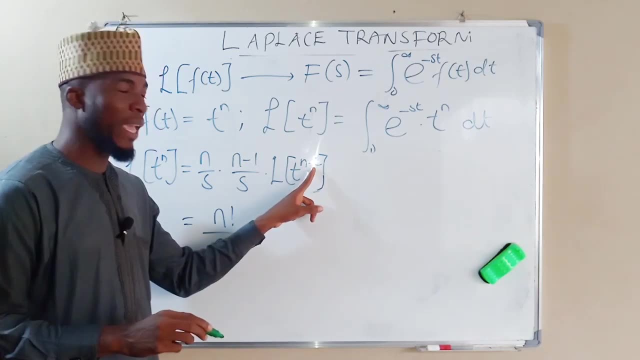 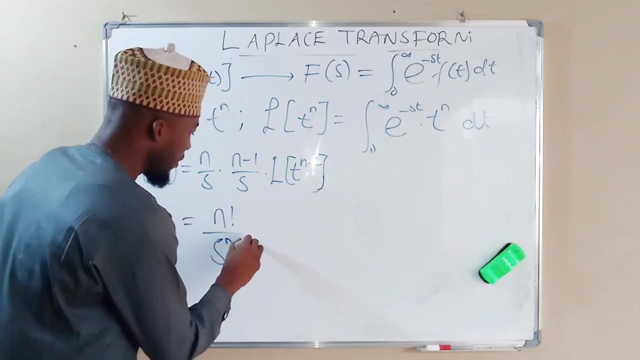 So this is n factorial all over s times s times s up to s to the power of n, because the last number is going to be n, Which is n minus n is 0, and t to the power of 0 is just 1 times the Laplace transform of 1.. 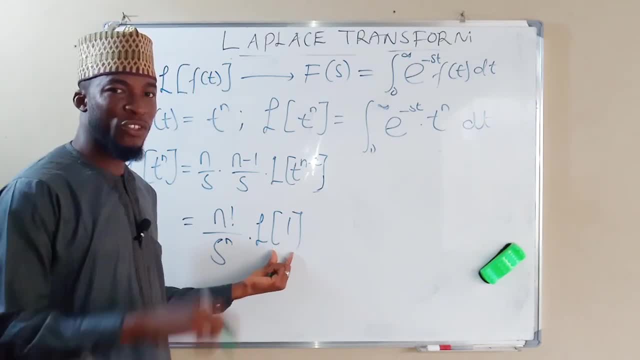 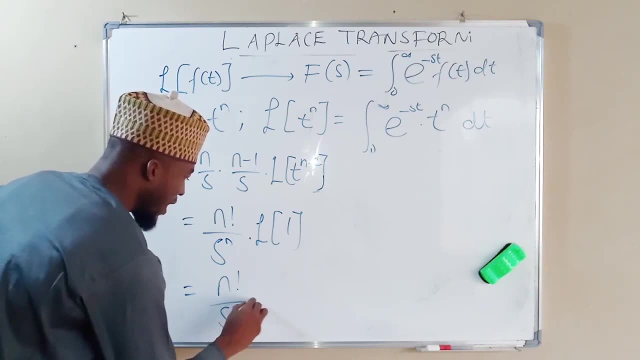 But previously we have seen that the Laplace transform of 1 is just 1 over s. So we say this is equal to n factorial all over s, to the power of n times 1 over s. This is equal to n factorial times 1.. 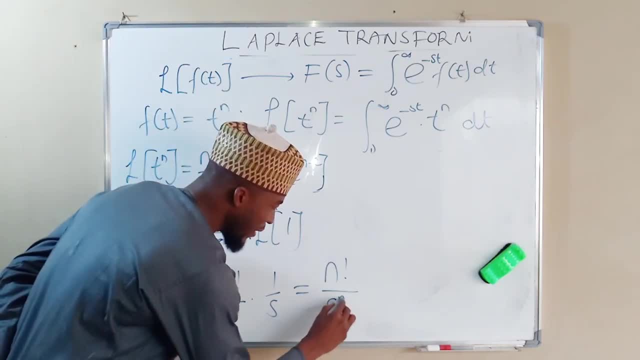 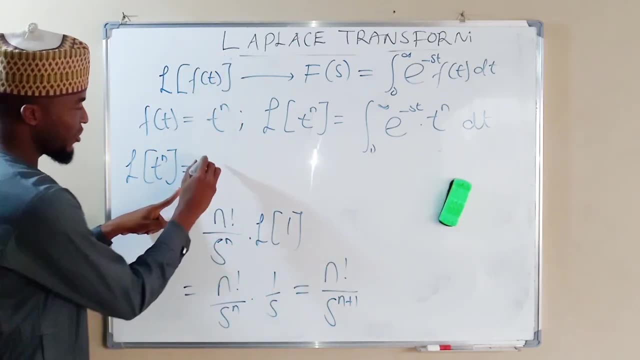 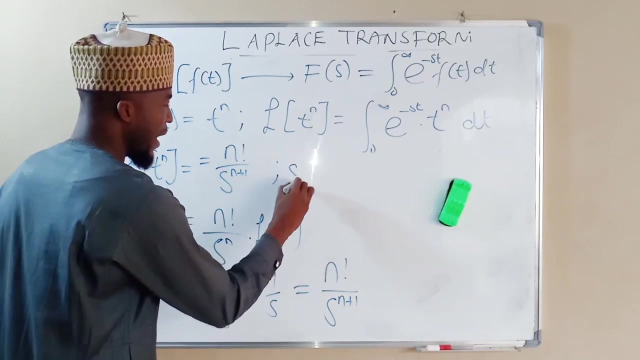 Then s to the power of n Times, s is just s to the power of n plus 1.. We can see that clearly. the Laplace transform of t to the power of n is just equal to n factorial divided by s to the power of n plus 1 for s greater than 0.. 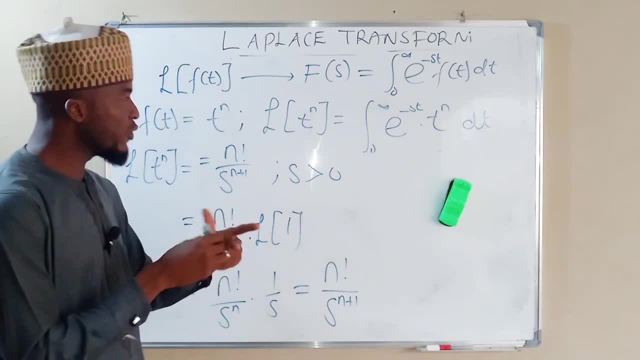 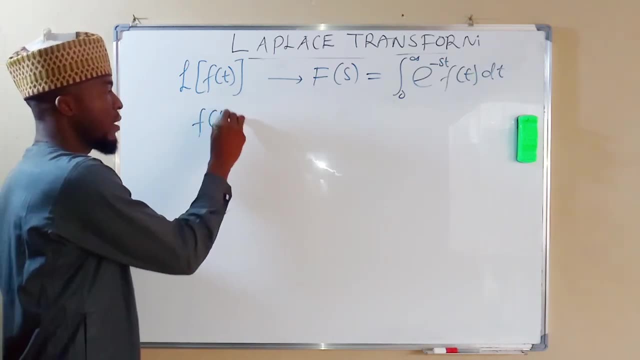 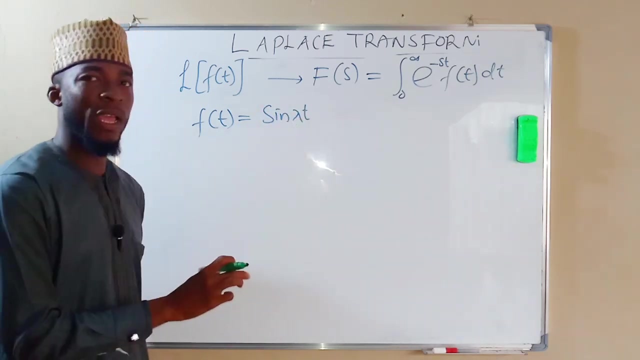 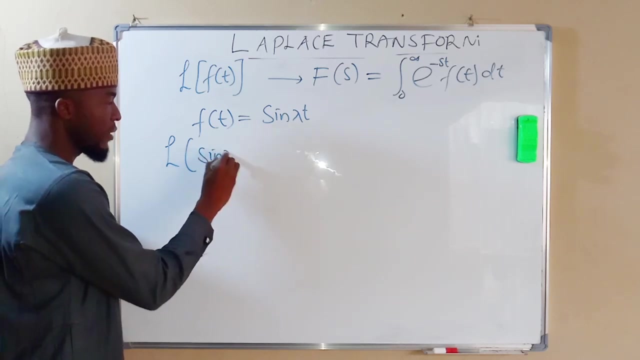 So now we have obtained the third equation, Now let us look on to the fourth equation. Now suppose f of t Equals sine lambda t for any constant lambda. The Laplace transform of this function in sine lambda t will now be equal to: 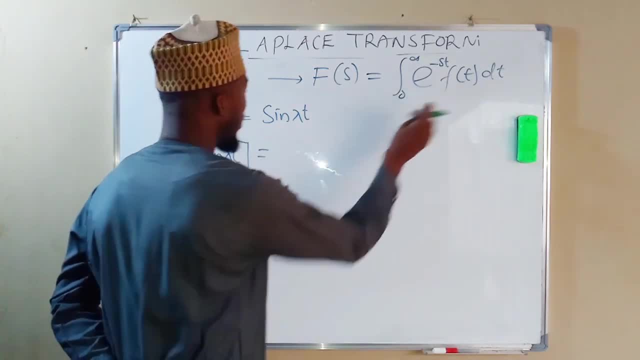 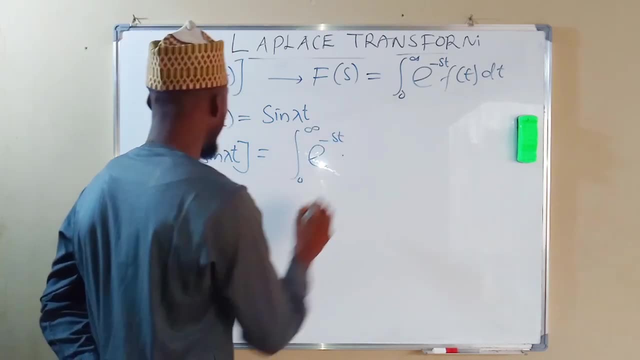 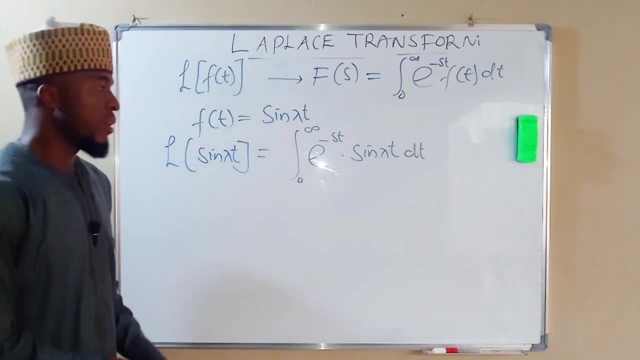 Because now we want to transform this into a function of s. I am going to apply this principle 0 to infinity of exponential negative st Times. the function which is sine lambda, That t with respect to t. Here we have to apply integration by parts. 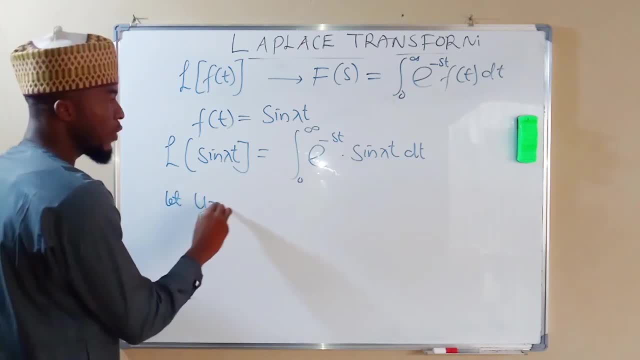 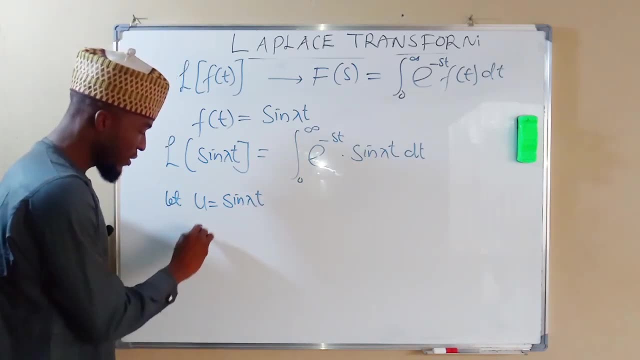 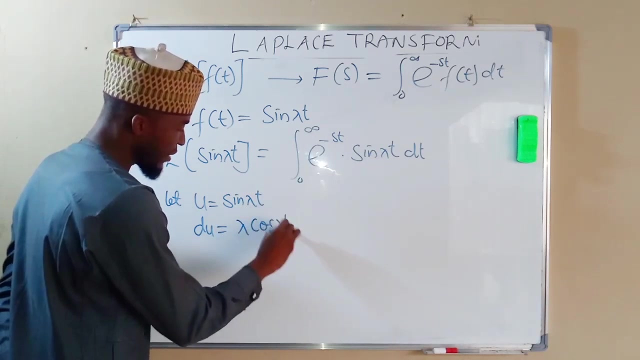 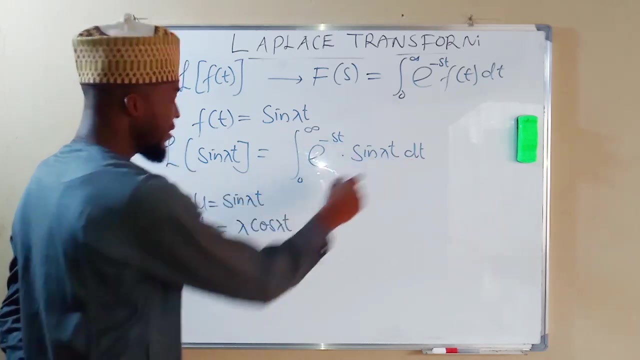 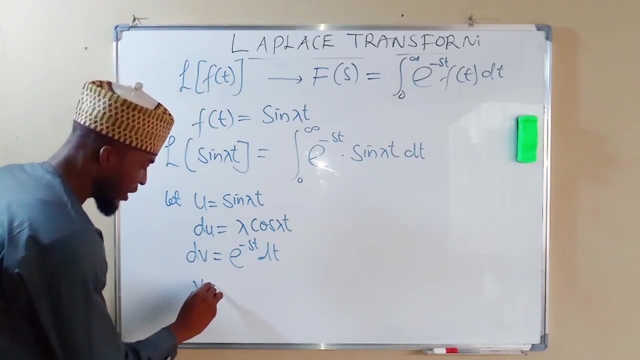 So let u equals to sine alpha t. If we differentiate u with respect to t, Du equals to lambda cos, lambda t Dv, Which is now going to be exponential negative st dt. If we integrate this, we are going to get v, and here negative 1 over s. 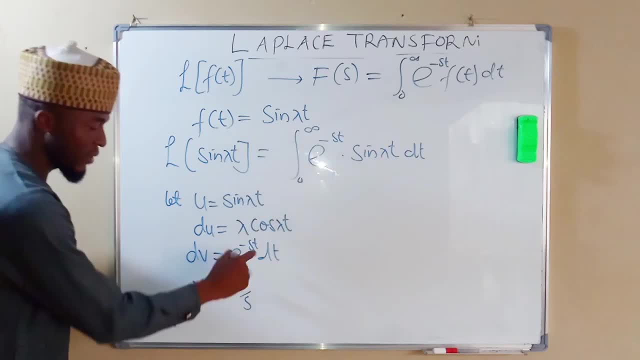 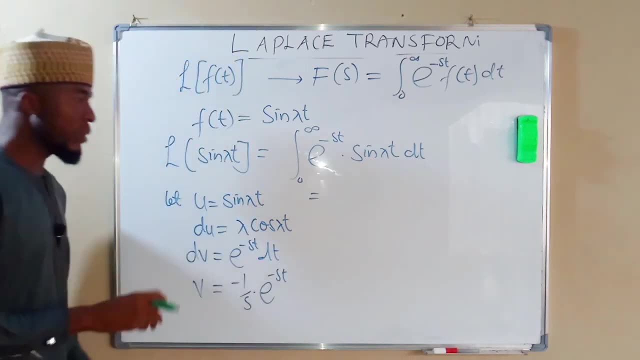 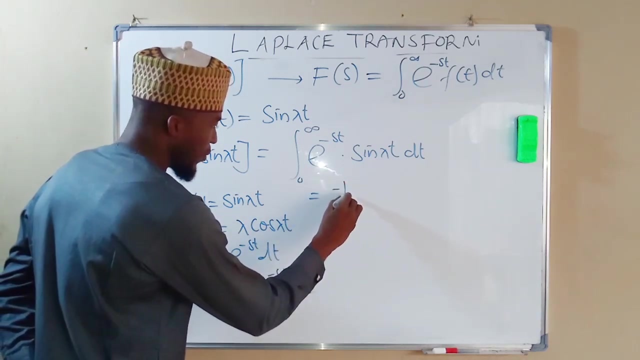 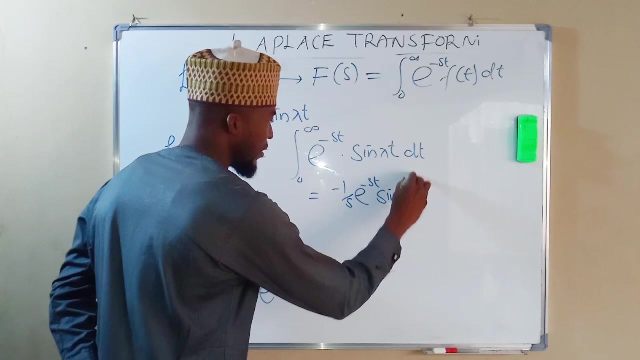 Because we have to take 1 over the derivative of this index times exponential negative st. Okay, now we are going to substitute- The first term is uv u and v? u is negative. 1 over s exponential negative st sine lambda t from 0 to infinity. 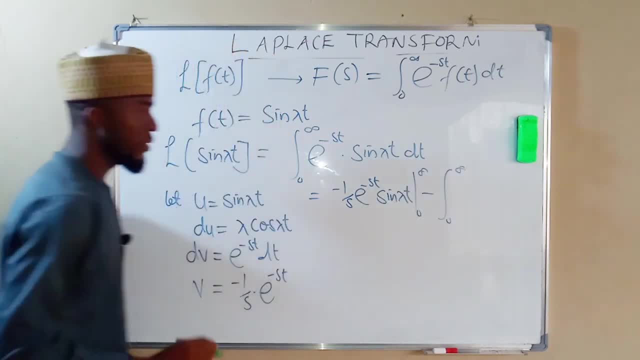 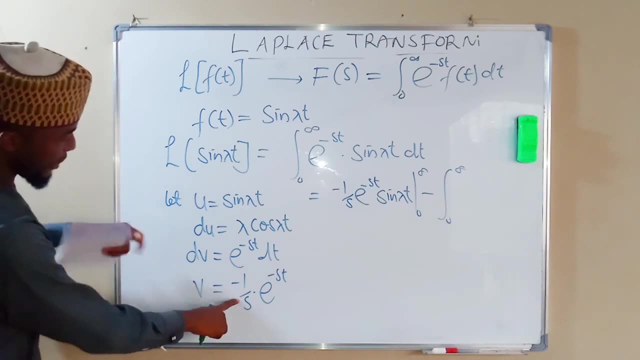 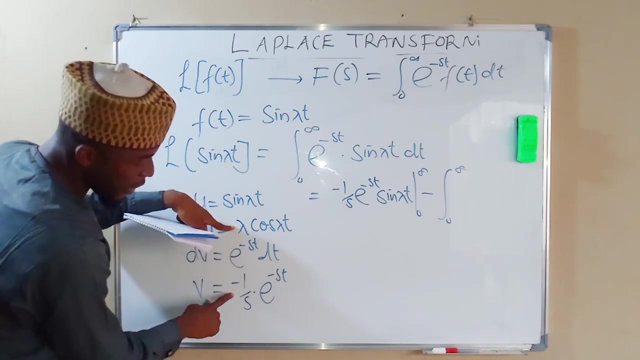 Minus the integral from 0 to infinity of vdu, We have v and we have du here, But they have a constant which is lambda, And here we have negative 1 over s. So we are going to multiply them together. 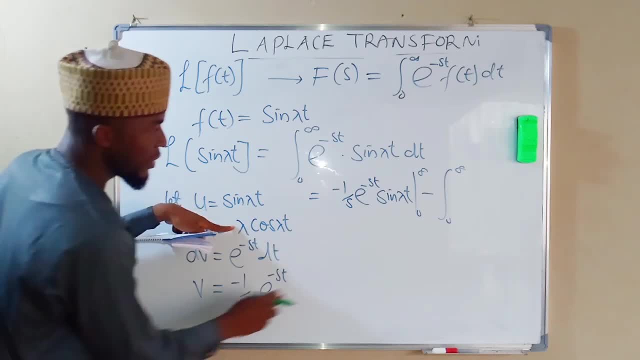 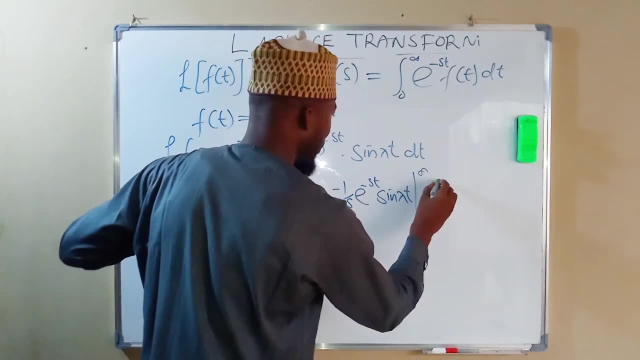 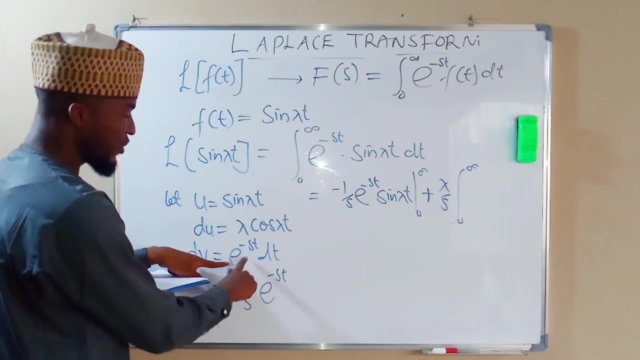 Which is going to be negative. lambda over s. If we multiply this negative with that negative, we are going to get positive. So let us factor out: lambda over s, Then integral from 0 to infinity of what is left. exponential negative st. then cos. lambda t. 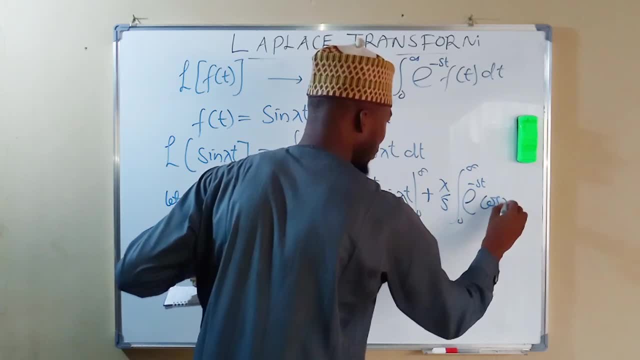 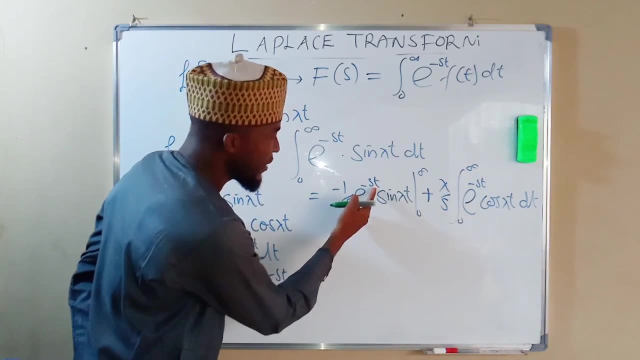 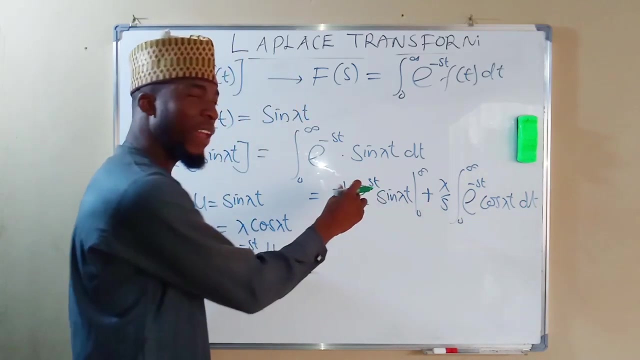 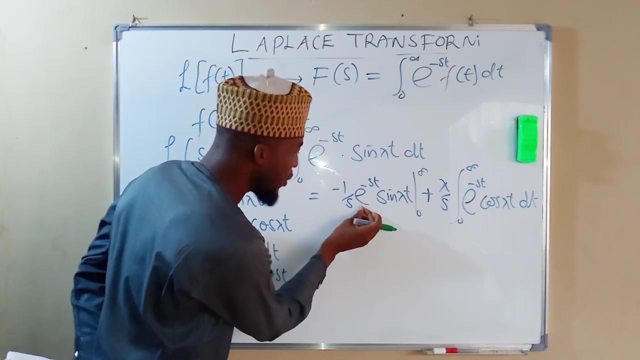 Exponential negative st, cos, lambda, t, dt. Let us substitute our upper and the lower bound. If we set t to be a number closer to infinity, we are going to get a negative infinity here And that number very close to infinity. If we take this exponential rest of the power of that number, we are going to get 0 here. 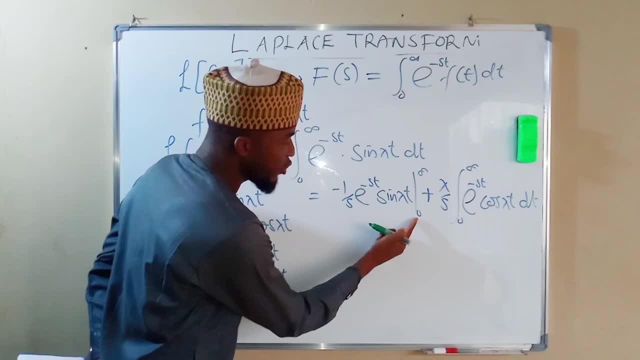 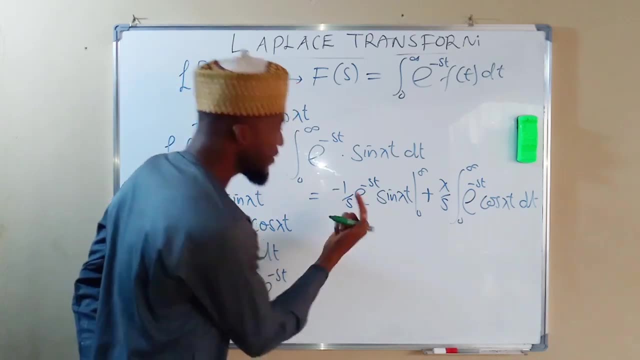 So 0 times the whole of this will make it 0.. And if we substitute t for 0, we are going to get sine 0. And sine 0, you know, is 0. This will make it 0.. Therefore, the whole of this will be 0. 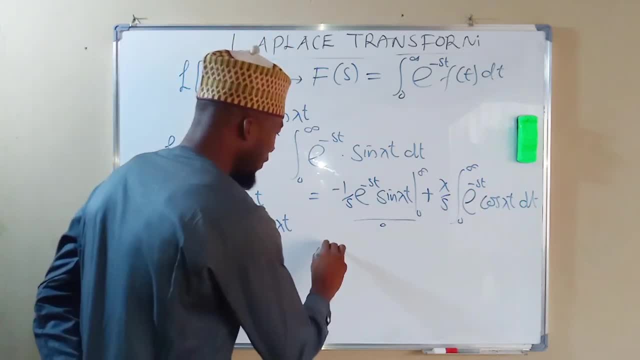 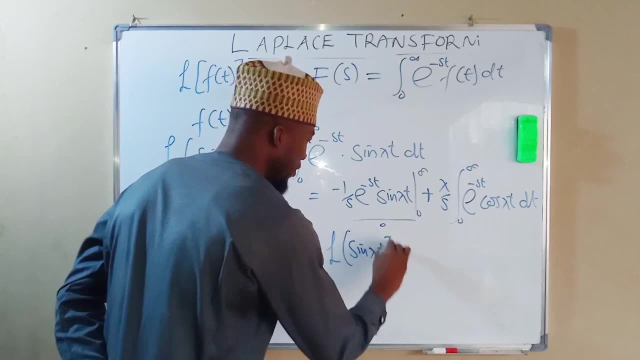 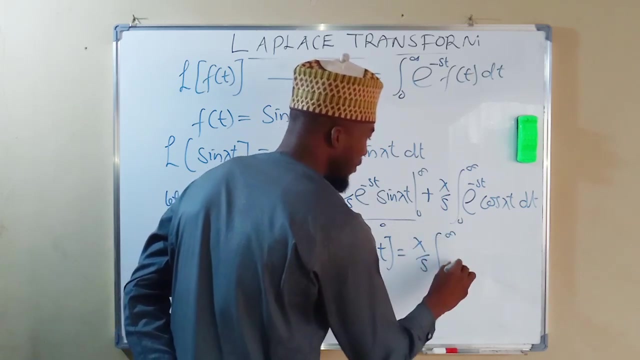 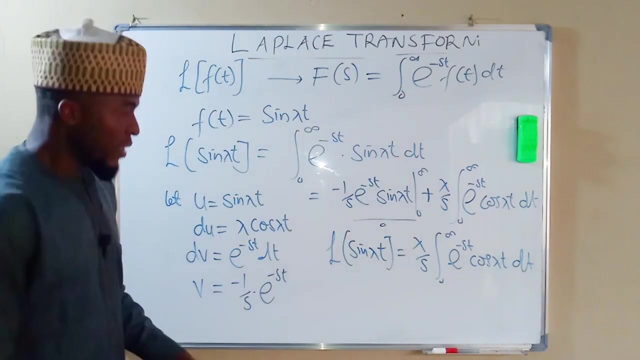 We only have this left. So we say the Laplace transform of sine lambda t will now be equal to lambda over s, The integral from 0 to infinity of exponential negative st cos lambda t, dt. So this is what we have. 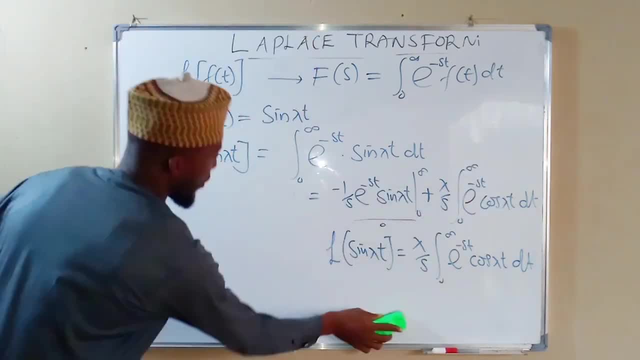 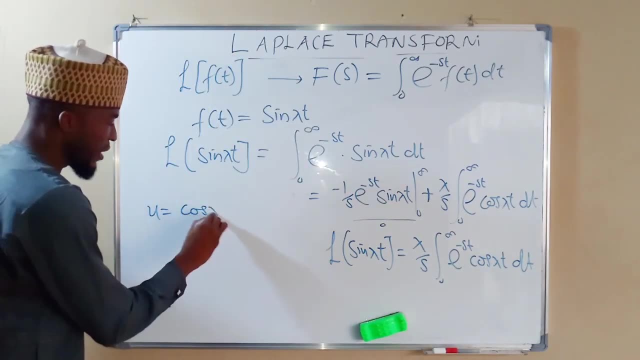 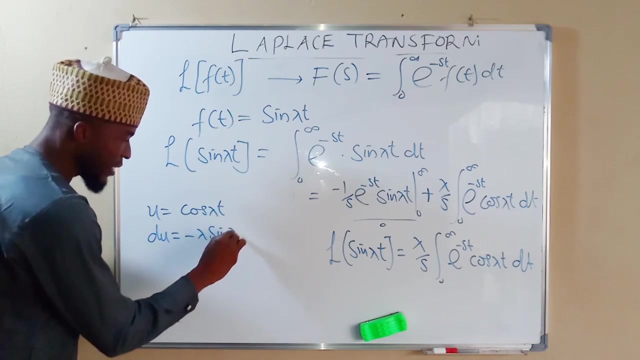 We want to now integrate this function again. Let's set cos lambda t to be our u. Let u equal to cos lambda t. The? u will now be equal to negative lambda sine lambda t. Then we set exponential negative st dt as our dv. 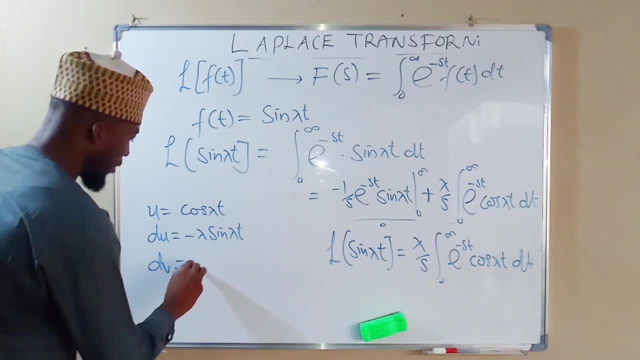 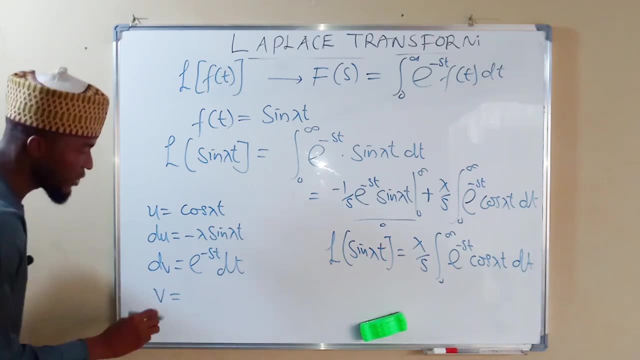 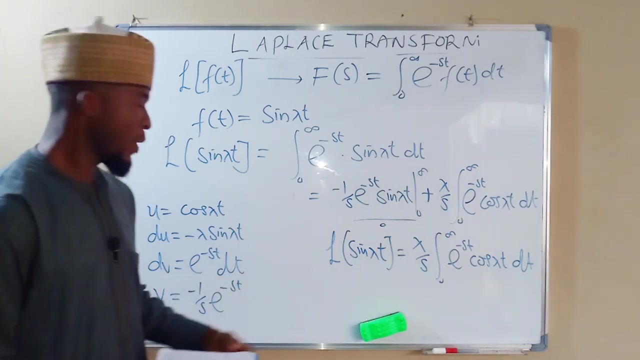 dv will now be equal to exponential negative st dt. To integrate this, we get v, And to the right hand side we have negative 1 over s exponential negative st. So we are going to substitute this back into that one. 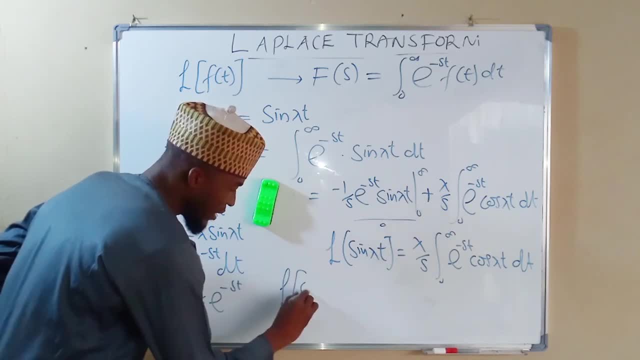 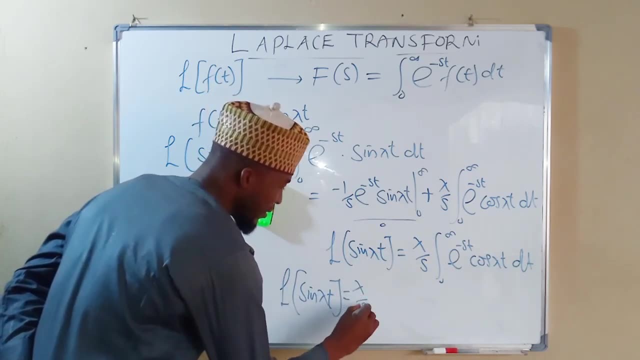 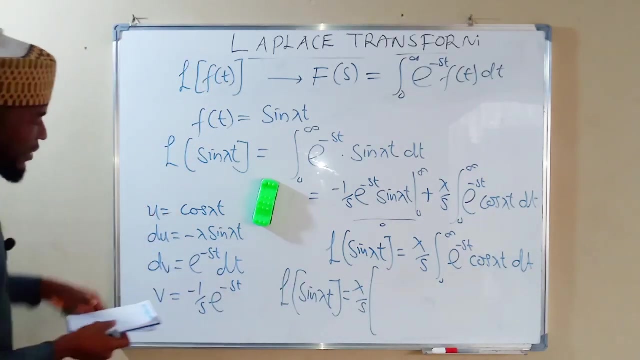 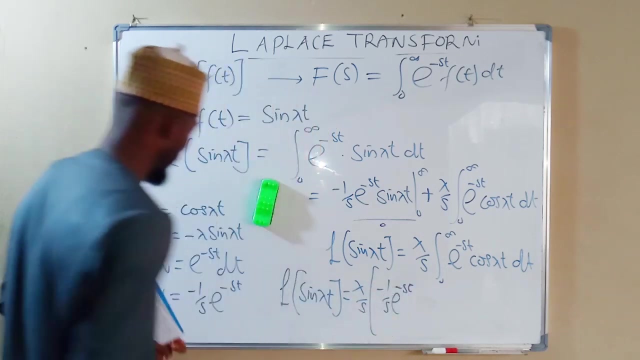 Therefore, the Laplace transform of sine lambda t will now be equal to this lambda over s times uv. This is u and this is v. We have negative 1 over s exponential negative st cos lambda t. This is the first term. 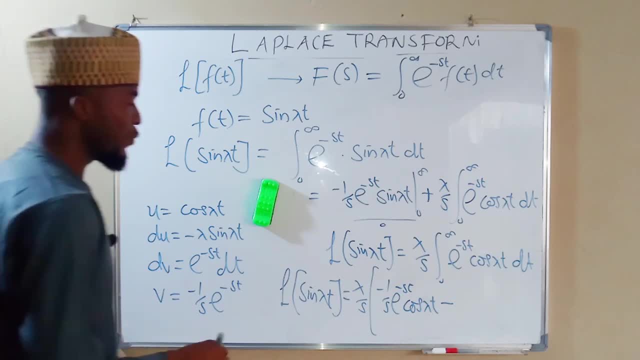 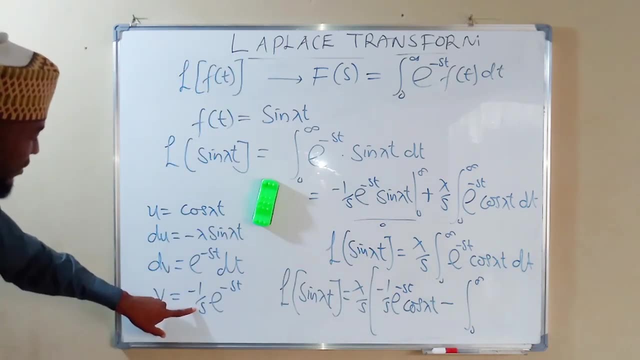 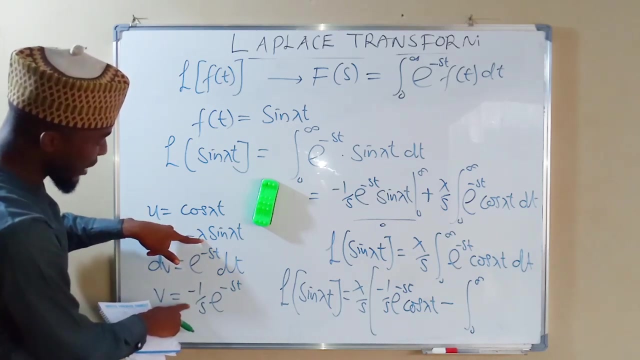 The minus, the integral of v du, The integral of v du, from 0 to infinity. Our v is this And du is this. Both of them have negative. If we multiply them we get positive. So we have constant lambda and 1 over s which we want to factor out. 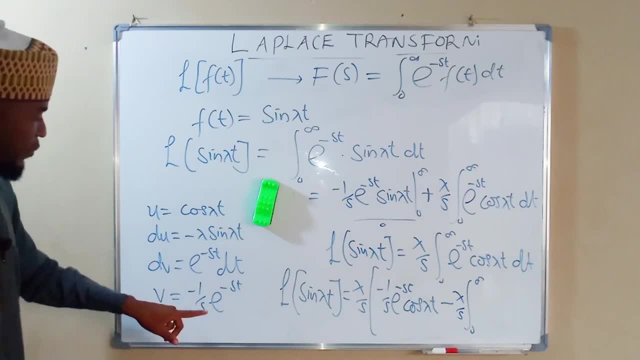 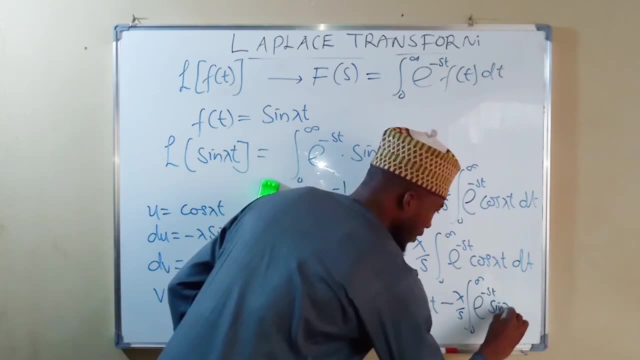 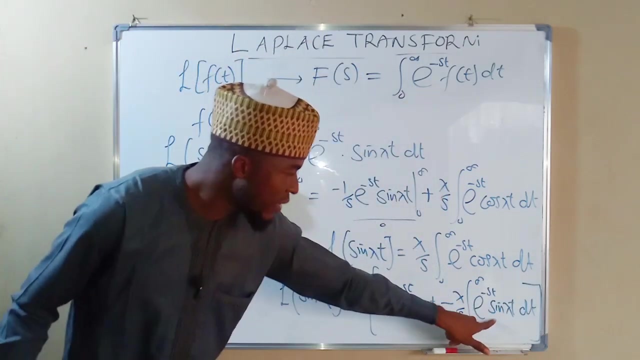 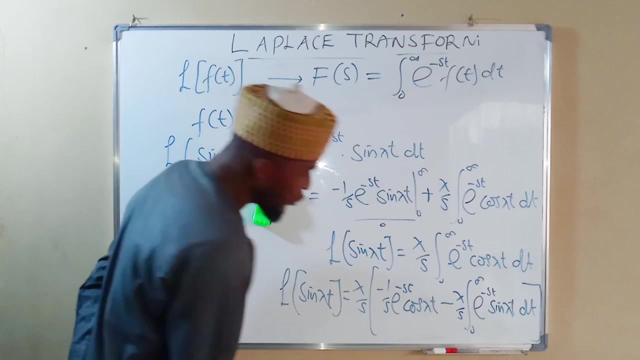 Lambda over s And inside we are going to have exponential negative st, then sine lambda t dt. This is what we have, But if you look at this, it's just The Laplace transform of sine lambda t. So what we are going to do, we are going to take the limit of this from here to here. 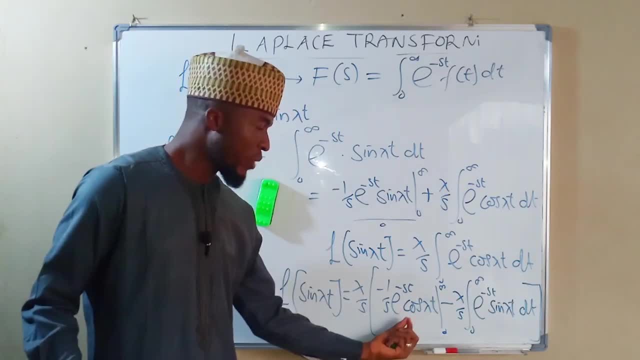 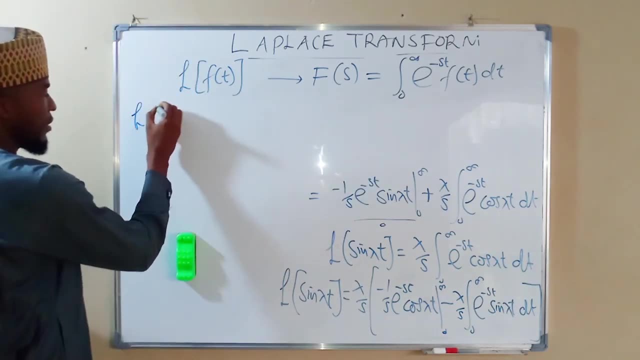 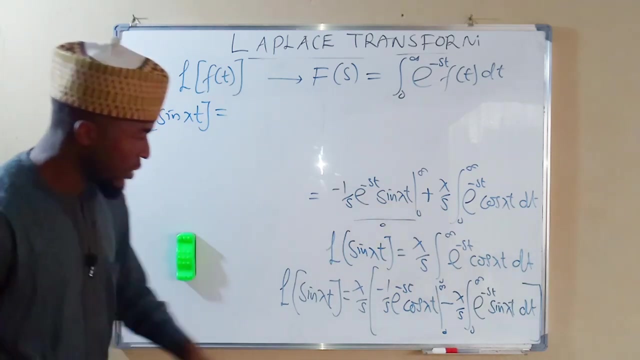 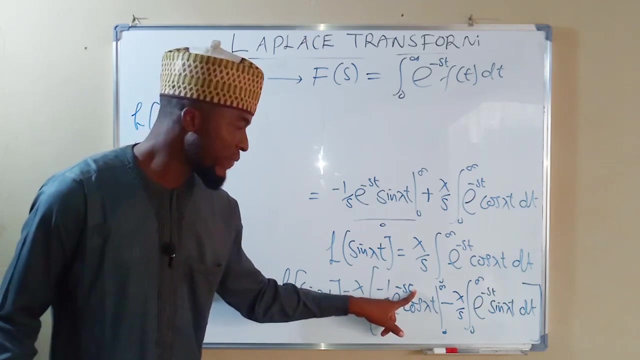 Since we have not finished integrating this, But since we are done with this, we can substitute the lower and upper bound here. So now let us move on. So the Laplace transform of sine lambda t will now be equal to: If we set t to be a number closer to infinity, this will become 0.. 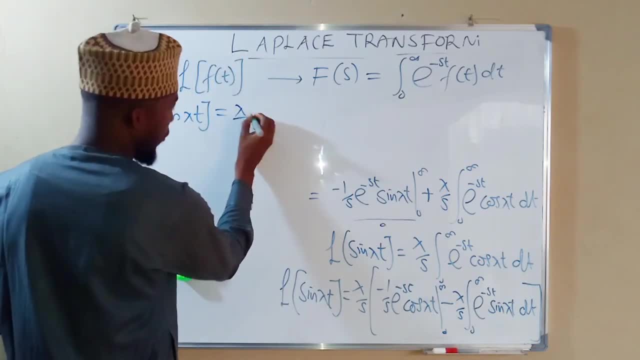 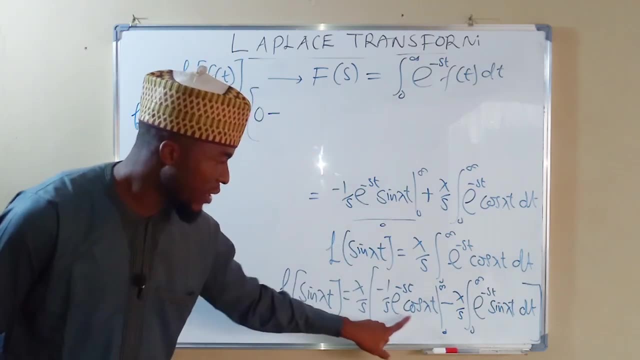 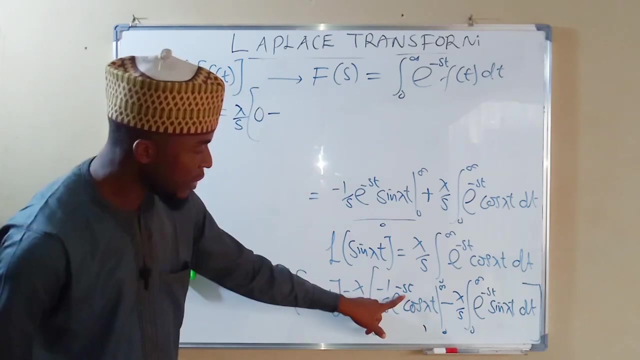 And this will become 0. So we have lambda over s minus. If we set t to be equal to 0, we have cos 0 and cos 0 is 1.. So we have 1 here. If we set t to be equal to 0, we are going to have exponential 0, which is 1 again. 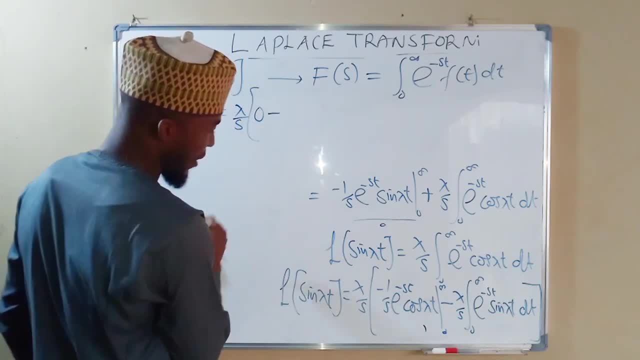 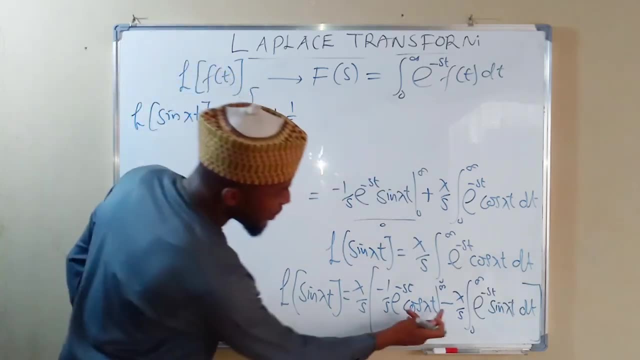 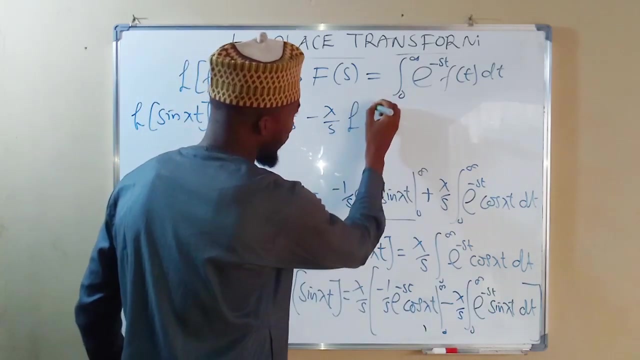 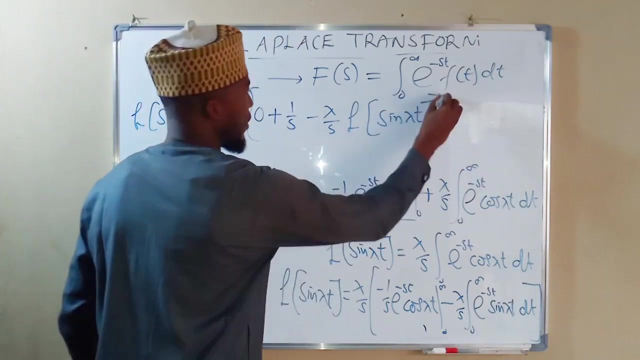 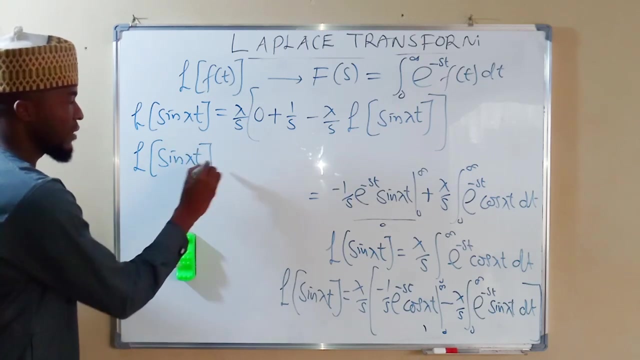 Times: this 1 is 1.. Times this: we are only going to have negative 1 over s, which will make it positive 1 over s. Then minus lambda over s times, the Laplace transform of sine lambda t. This will be equal to the Laplace transform of sine lambda t equals to this time. this will make it 0.. 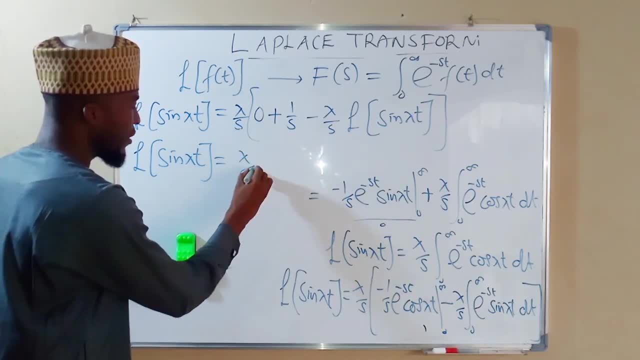 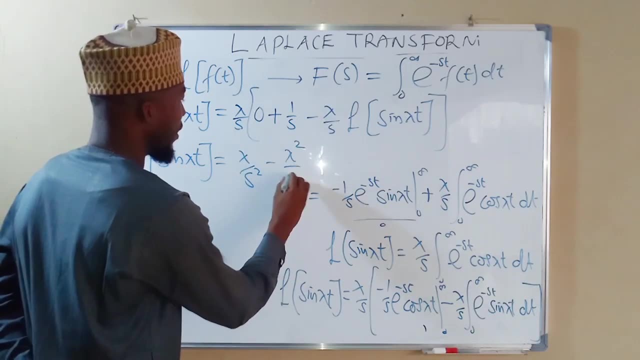 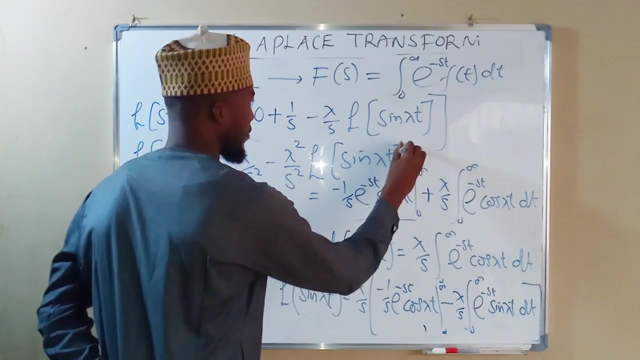 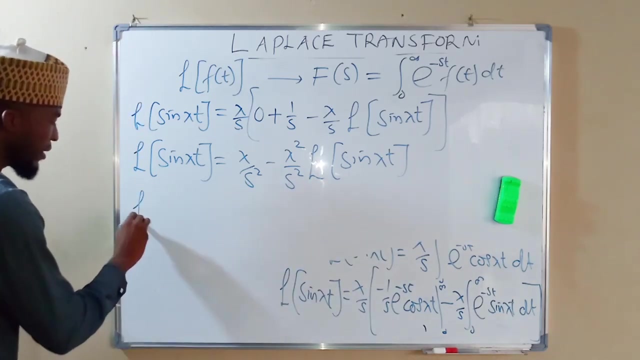 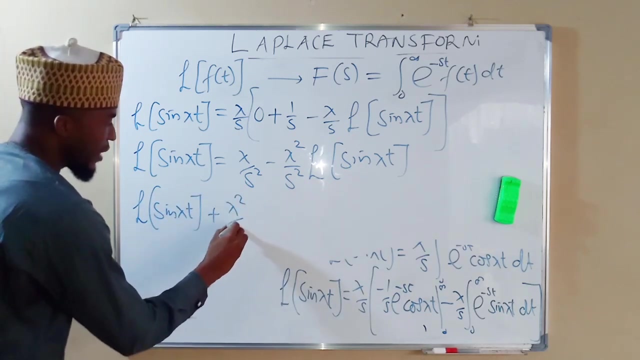 This time this will make it lambda over s squared, minus. this time this will make it lambda squared over s squared. Laplace transform of sine lambda t. Now, since we have common terms, we can bring this one backward, so that we have Laplace transform of sine lambda t plus lambda squared over s squared. 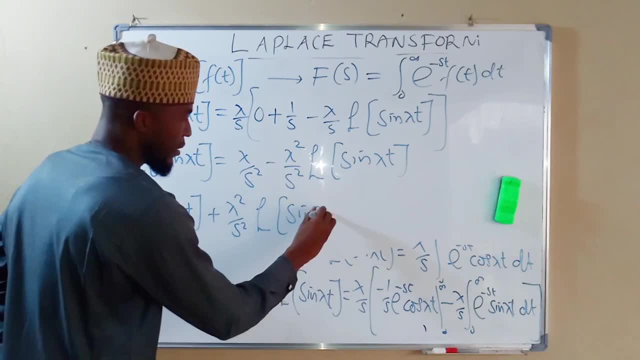 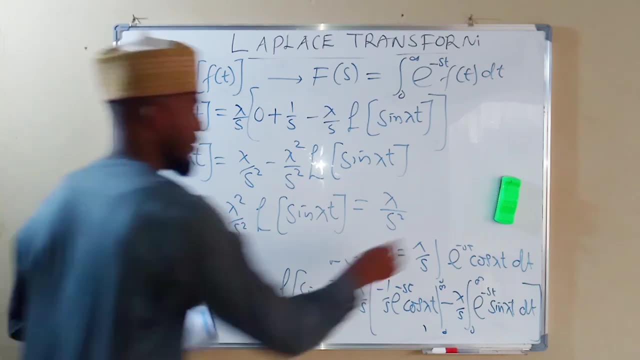 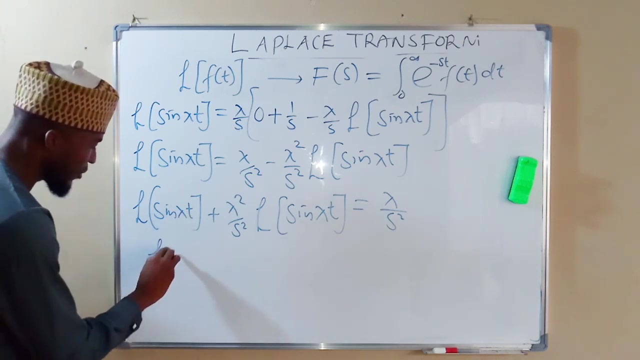 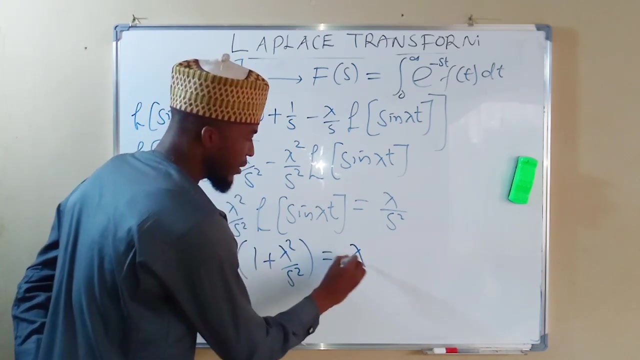 Laplace transform of sine lambda t, which is now going to be lambda over s squared. We can factor out the Laplace transform of sine lambda t times. here we have only 1, plus. lambda squared over s squared equals to lambda over s squared. 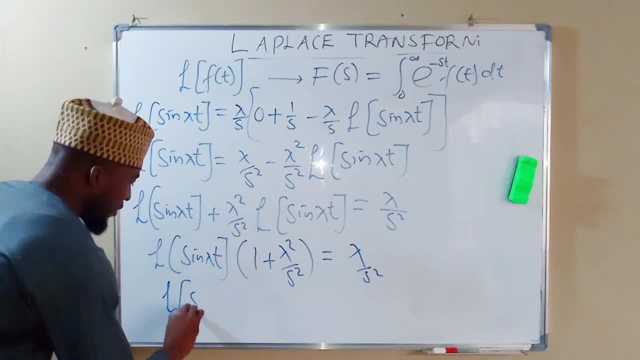 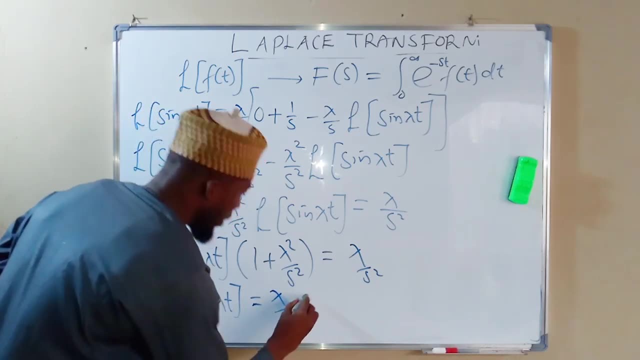 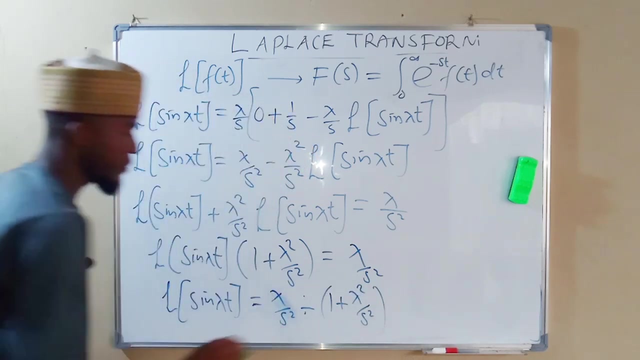 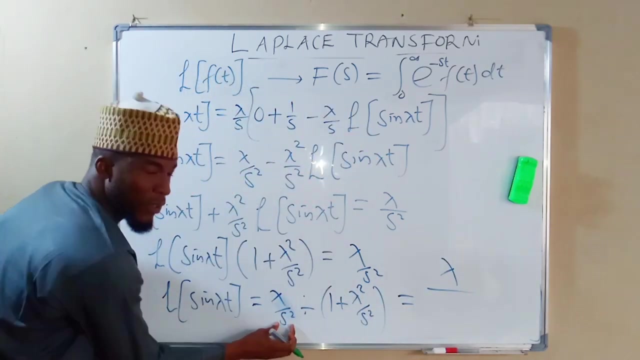 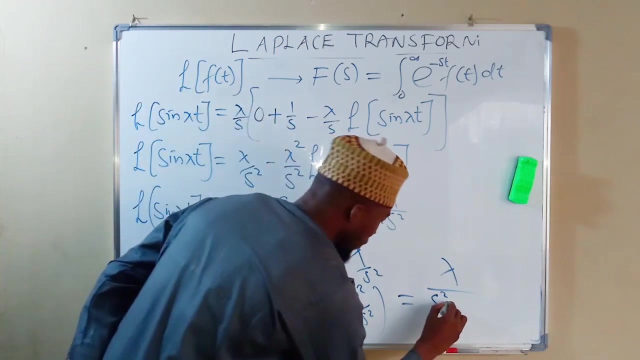 Therefore, the Laplace transform of sine lambda t will be equal to lambda over s squared divided by 1, plus lambda squared over s squared. This is going to be equal to this. lambda divided by s squared times. 1 is s squared s squared times. lambda squared over s squared is just lambda squared.